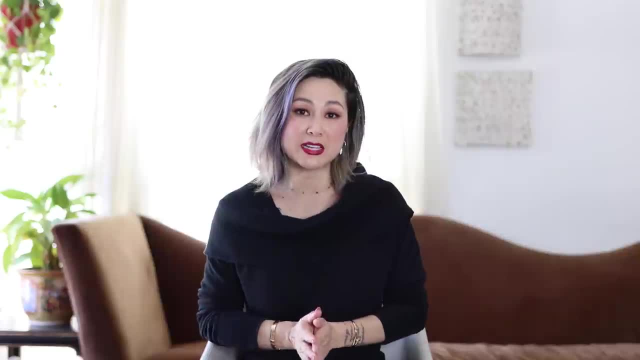 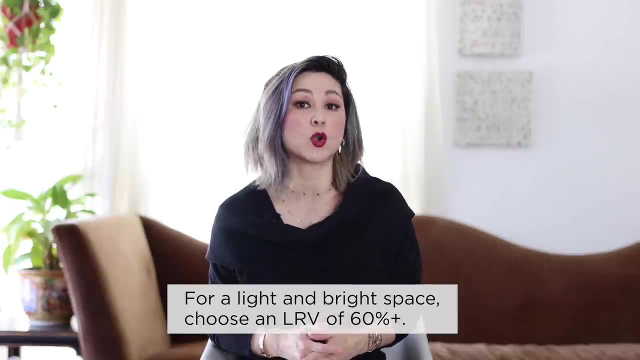 Is higher LRV better? That's really subjective and it all depends on your design direction. If you want a light and bright space, anything with an LRV of 60% or higher will suffice. For kitchens and bathroom cabinets, the LRV value of 80 plus is usually ideal. 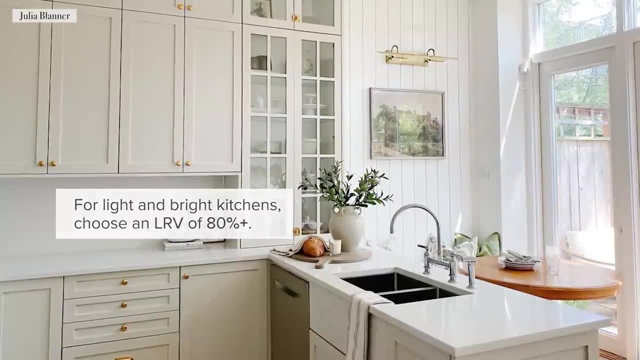 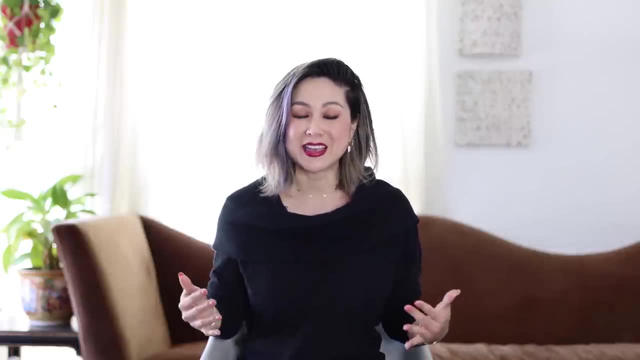 You can find the LRV value on the back of the paint sample or the paint chip. But, to be perfectly honest, I rarely check the LRV value of a paint color. nowadays, With my decades of experience with paint colors and samples, I don't really check the LRV value. 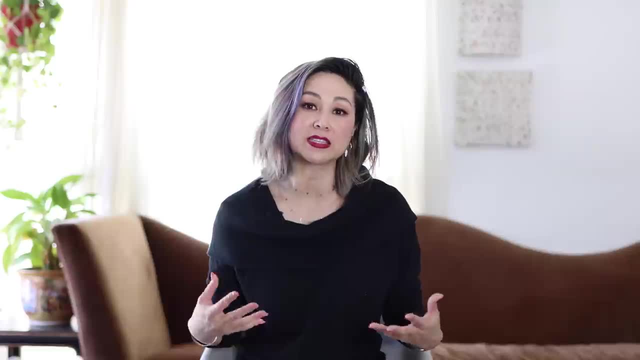 I can look at a color and know right away whether or not it's going to work in my client's space and for their conditions. With that said, let's dive right into my new favorite neutral paint colors for 2023, sectioned off into specific categories to make your search for the perfect. 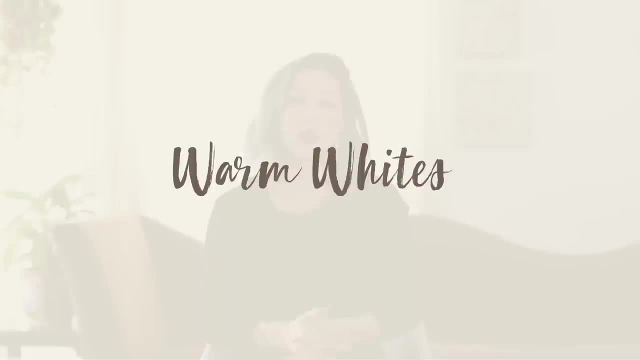 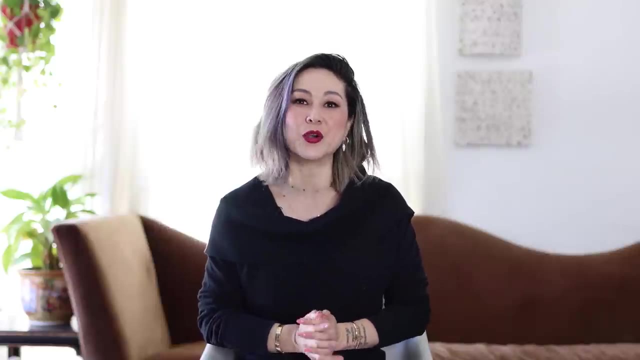 color easier and more efficient. Starting with warm whites, Chances are. if you see a really beautiful interior and the walls look white, most likely it is a warm white hue. Warm whites continue to be my reigning neutral because of the LRV value. So if you're looking for a 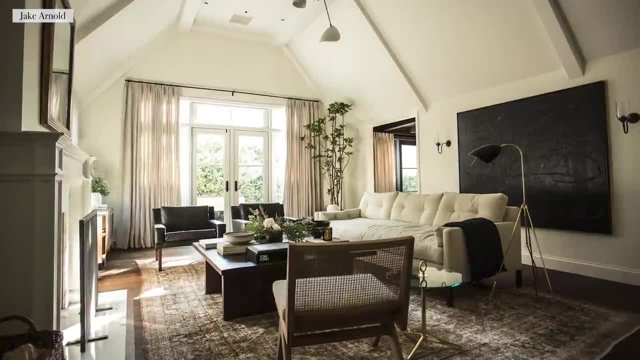 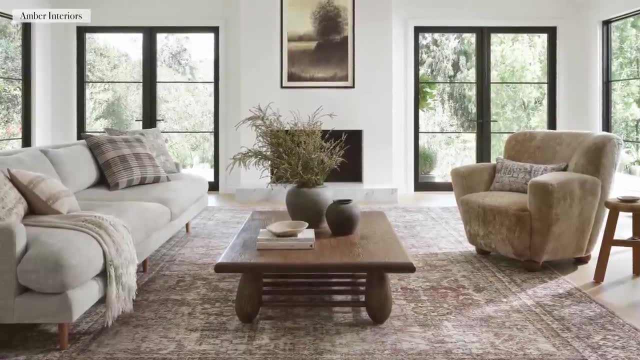 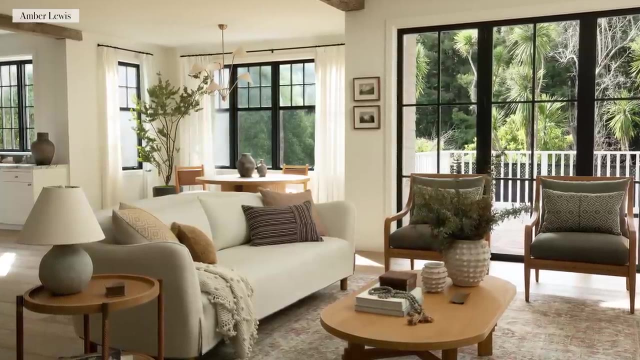 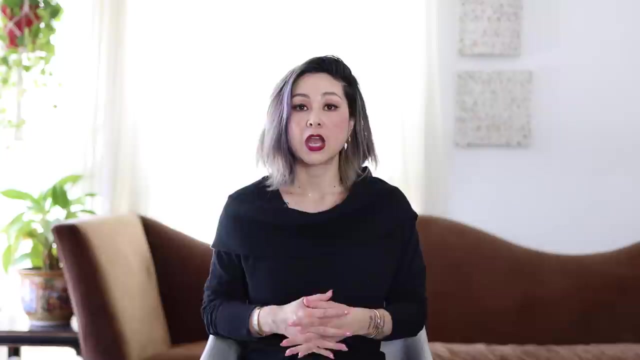 warm white hue. you can go ahead and check out the LRV value on the back of the paint sample sample. Warm whites are so versatile and with undertones of yellows, oranges and reds, you're sure to find the perfect warm white to suit your aesthetic and interior. Remember that a lot of whites can. 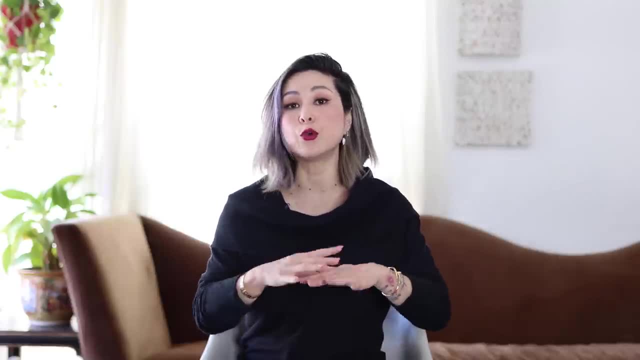 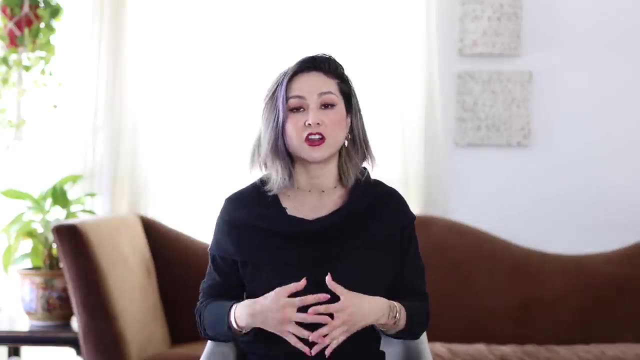 actually pick up the color that's being reflected in that light. So if you're looking for a warm white hue, you have a light-filled space with a lot of windows and that window is next to your courtyard or your backyard and there's a lot of greenery. there is a high probability that the 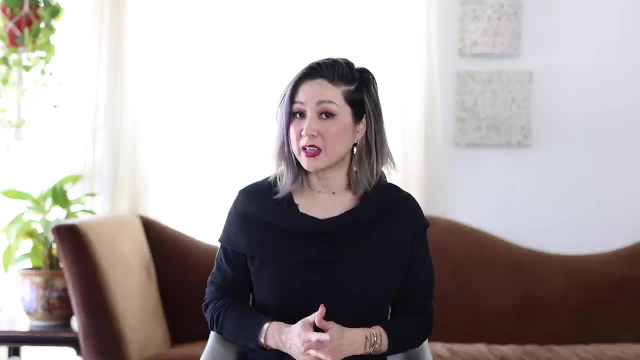 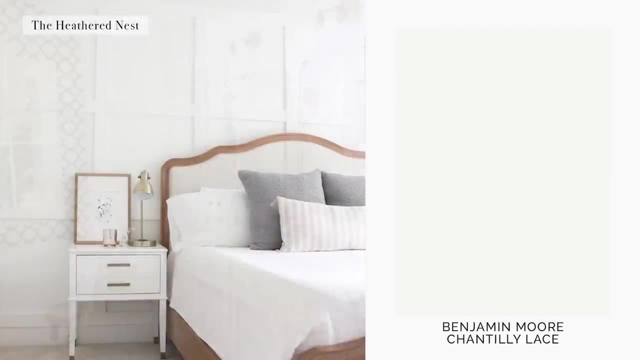 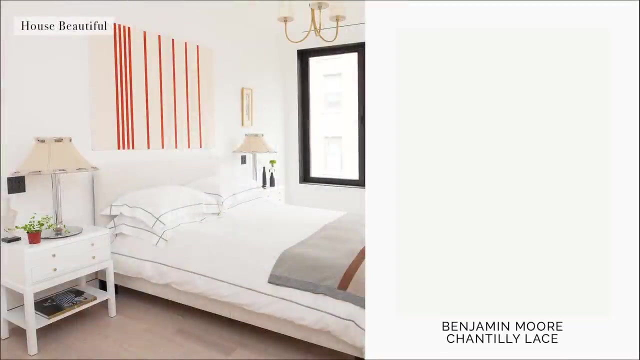 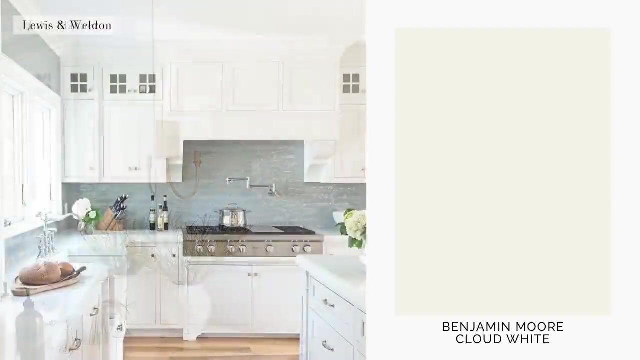 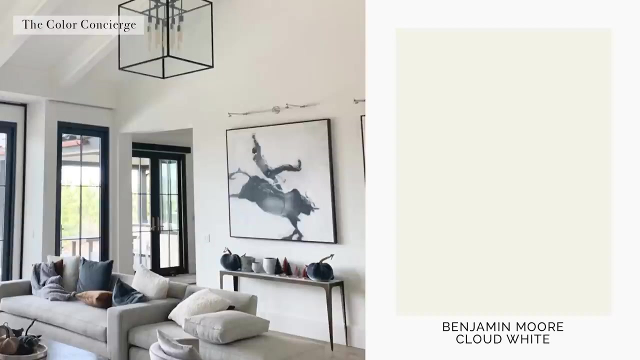 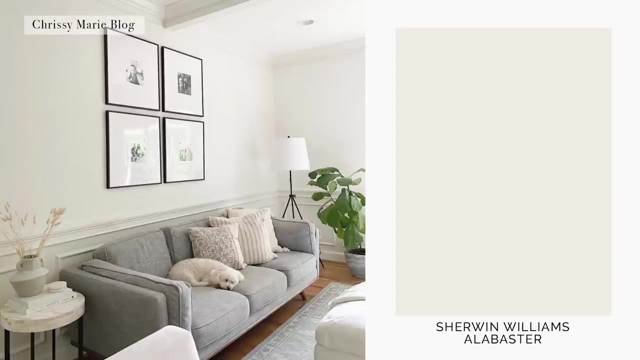 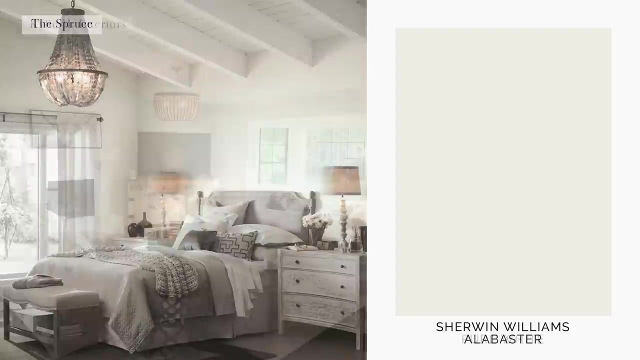 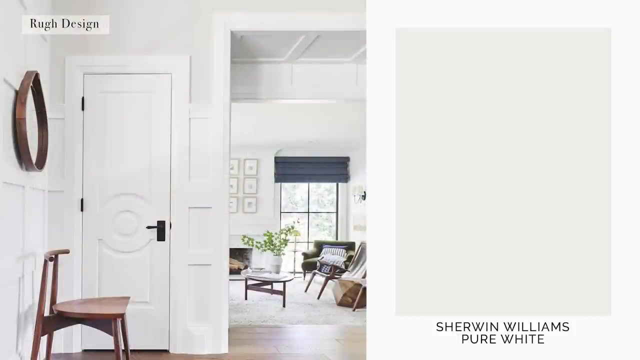 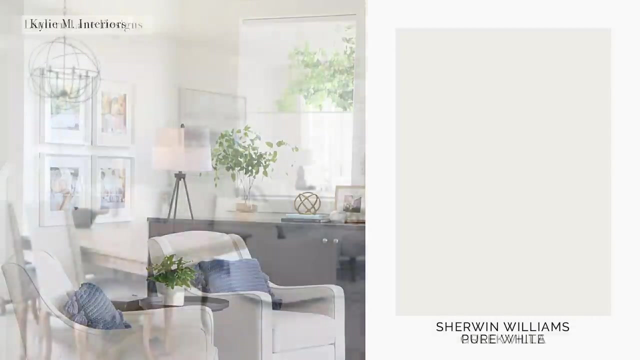 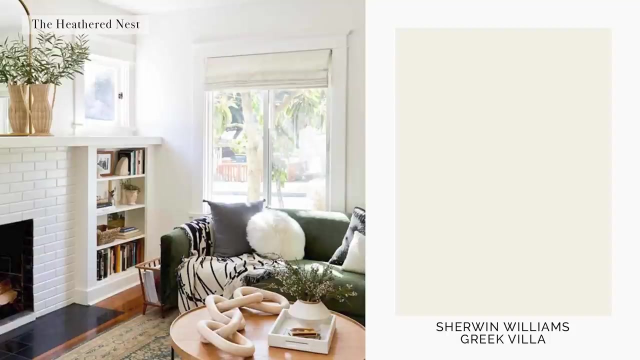 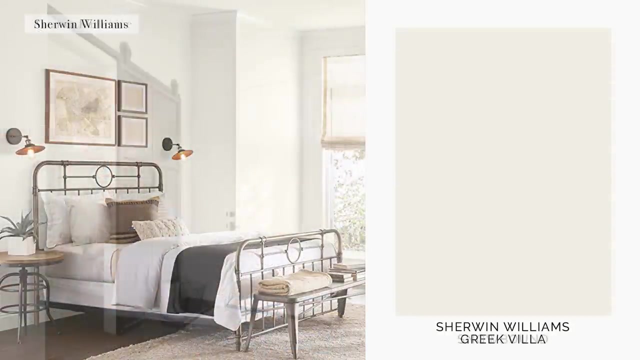 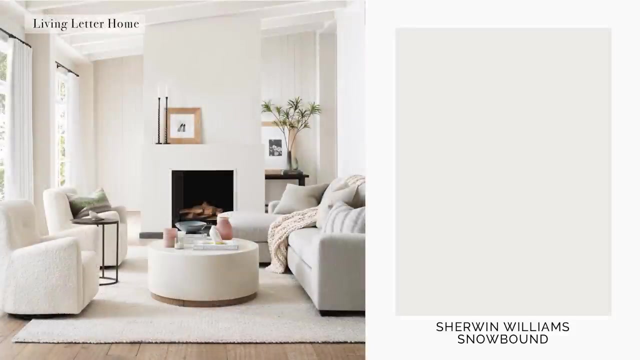 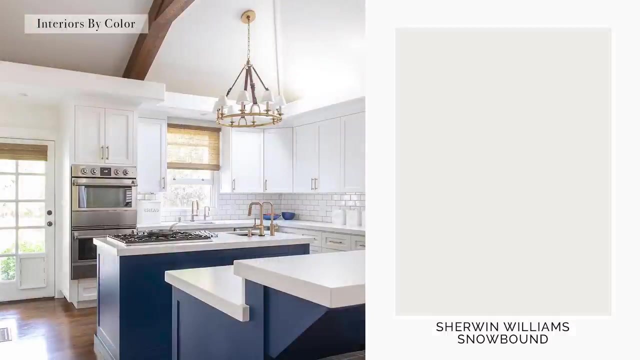 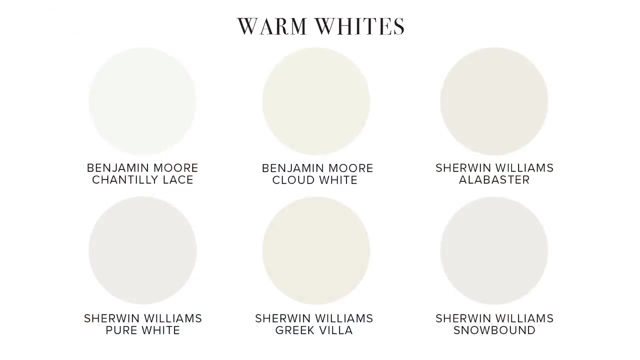 space will appear green as well, So definitely be very considerate of the white or warm white that you choose. I look forward to seeing you all in the next video. Thank you. See you then. Bye-bye, Thank you, Let's talk about warm creams. 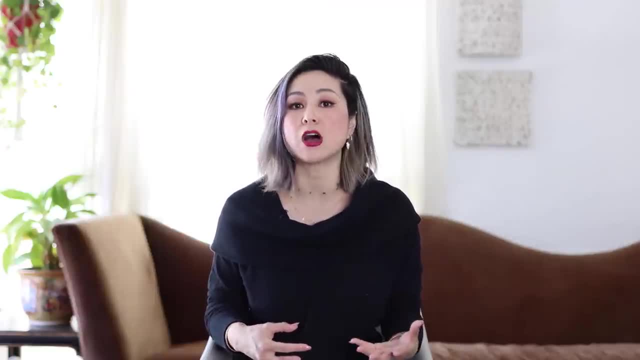 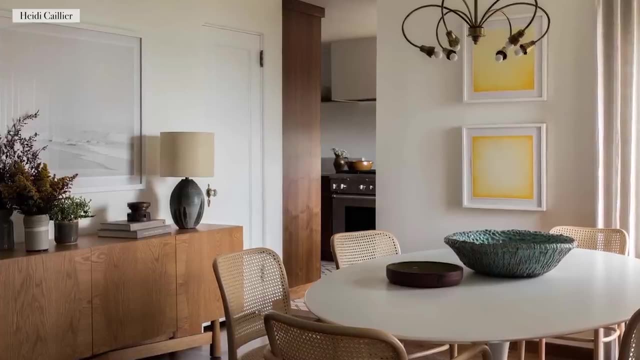 Cream is a very popular neutral paint color because it's a little bit softer and warmer than warm whites with a little bit more of a yellow undertone If you're looking to add just a tint more color while still reflecting a good amount of light. 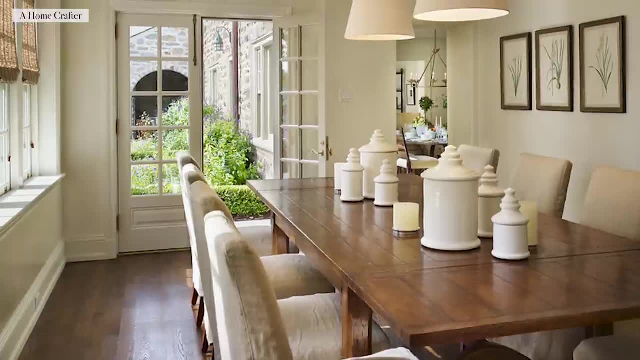 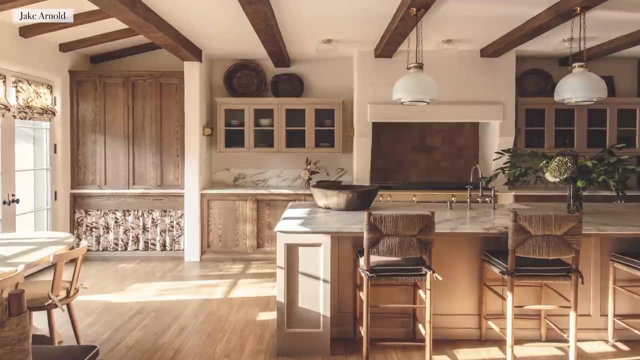 warm cream may be the right choice for you. If you have an affinity for cooler light sources, let's say 3000K or above, in your home, warm creams will warm up your space, But if you have warmer light bulbs in your home, 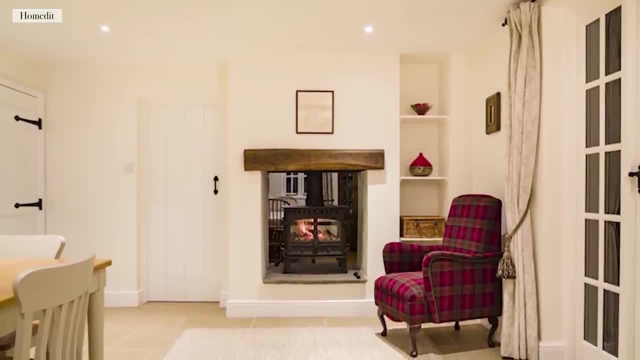 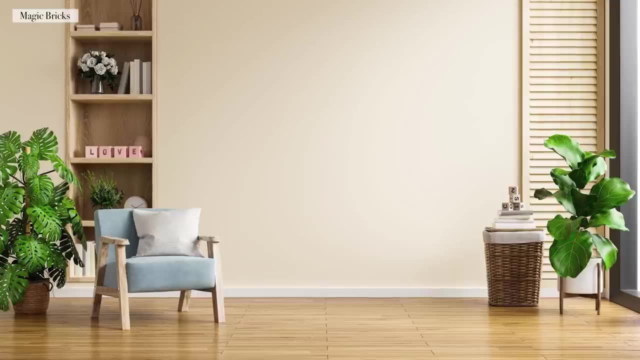 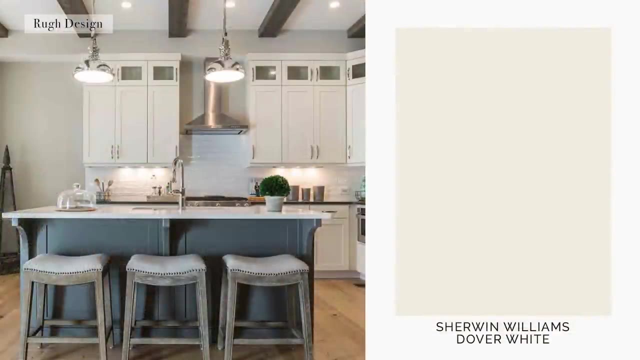 like 2700K or less, your space can look more yellow than preferred. So definitely test out multiple shades of cream. put them next to a white sheet of paper or your existing white trim to lock down the perfect warm cream hue. Thanks again for watching this video. 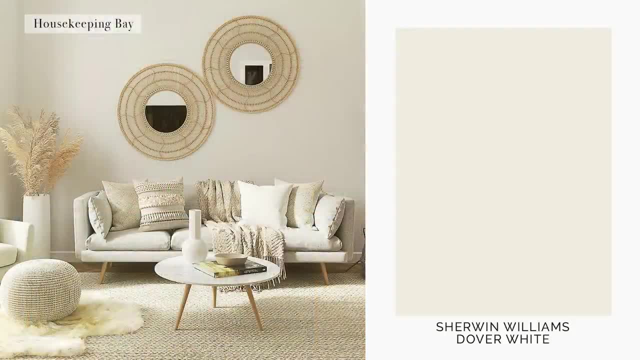 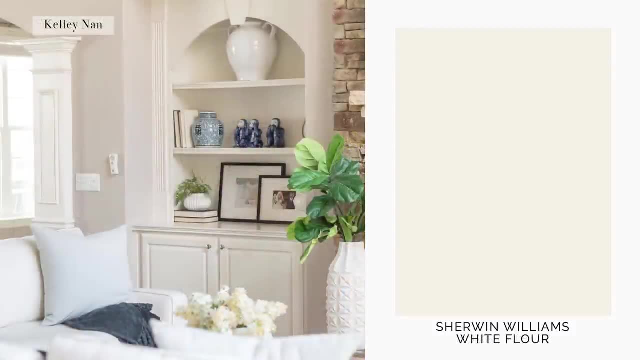 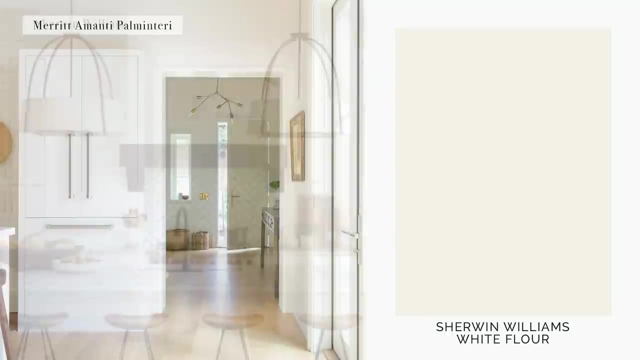 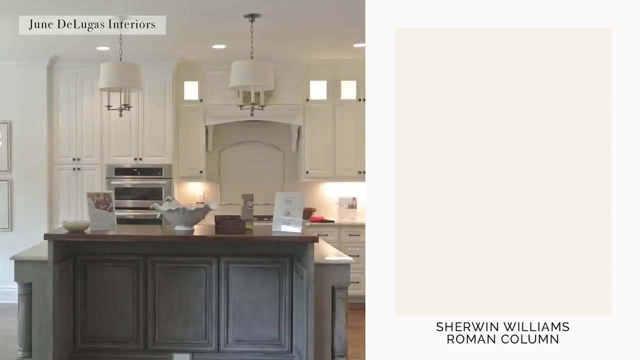 If you have any other questions, feel free to email me through the emailtowns at uscphamilycom. Thanks again for watching this video. Let's see how this works. Let's see how this works. Let's see how this works. 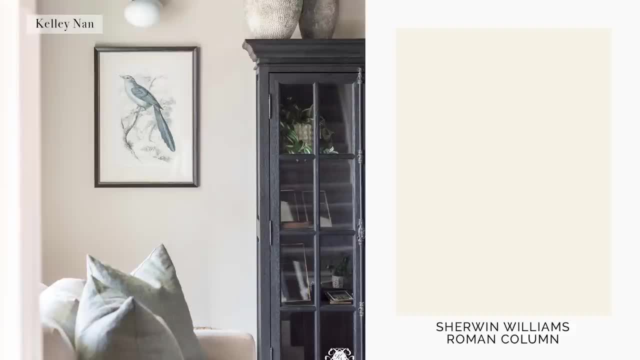 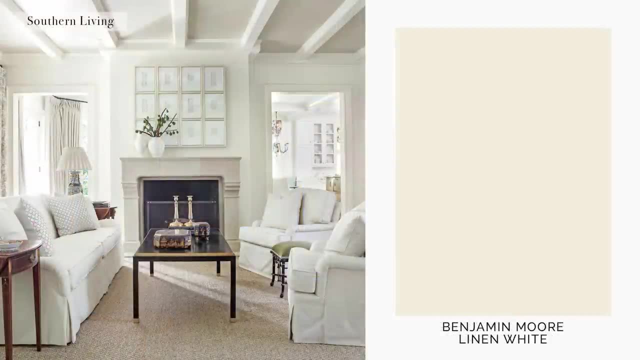 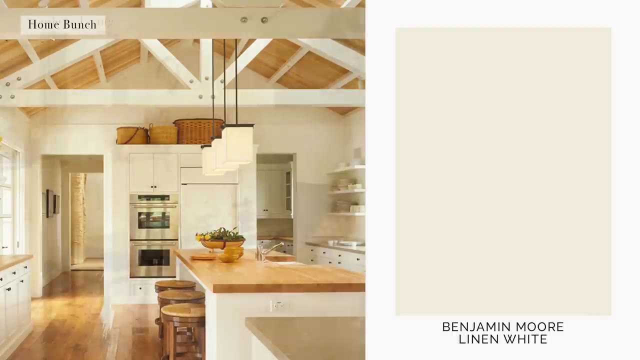 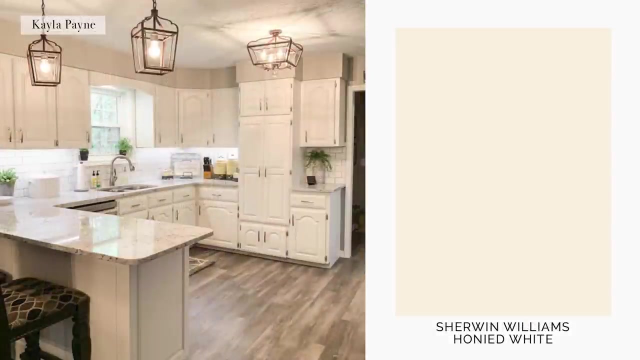 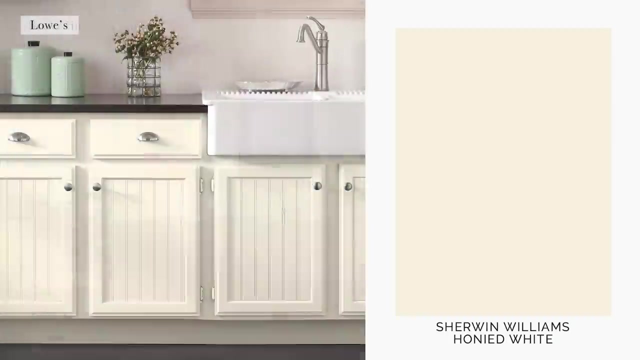 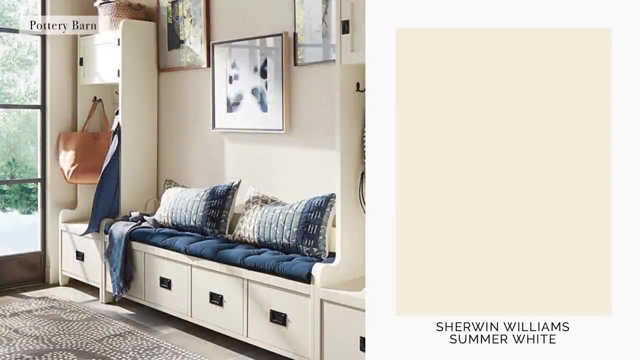 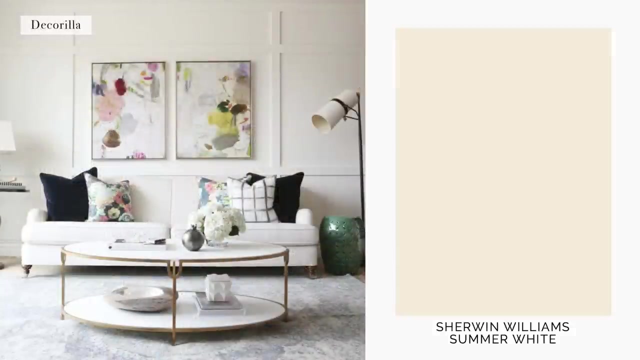 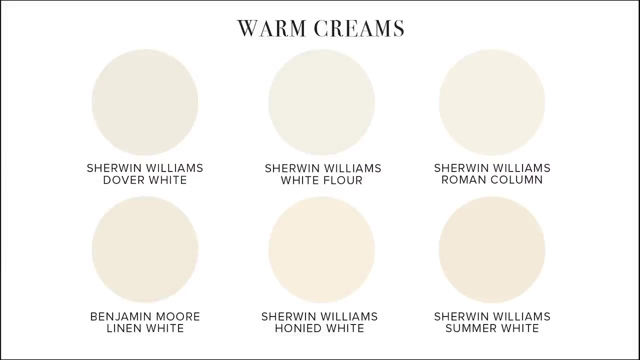 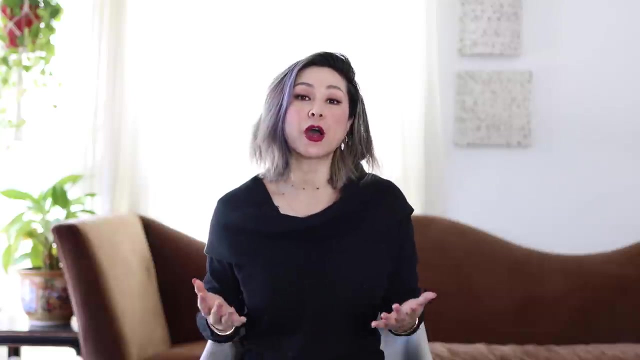 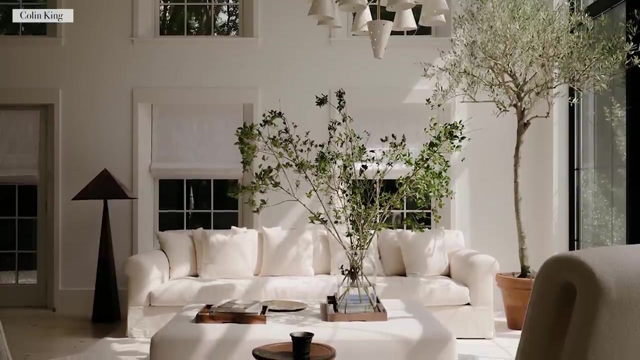 Thank you. Next we have my favorite warm off white grays. I talked about grays. I talk about grays here on the channel. quite often, Grays is simply a mix of gray and beige. I often consider it the perfect mix. 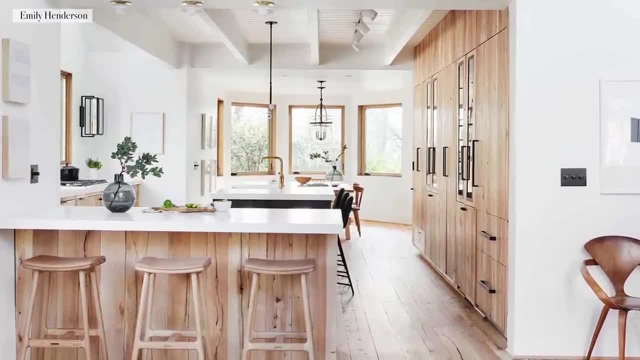 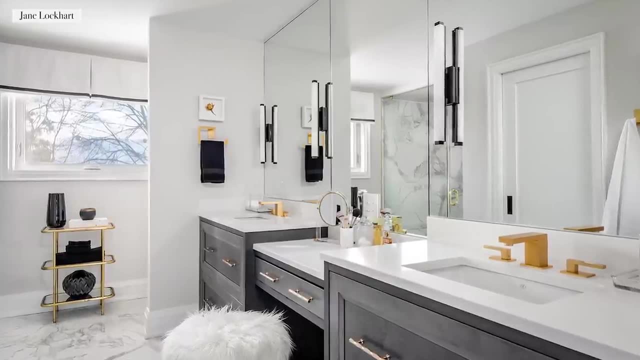 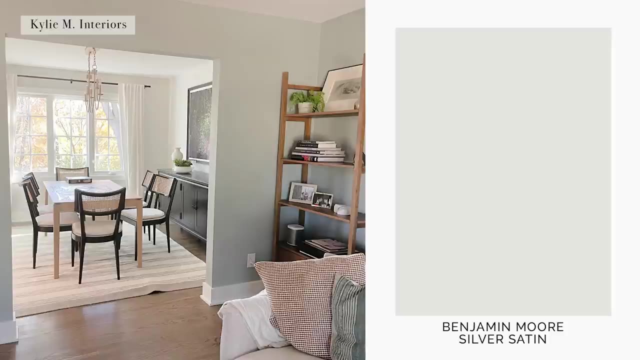 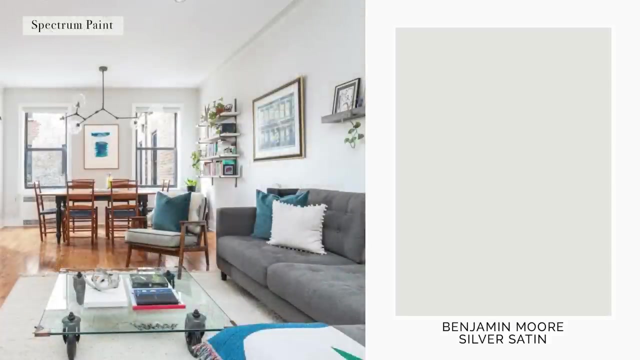 These have a hint of lavender in them and look equally as great in traditional interiors or more contemporary settings. Try pairing these wall colors with off-white trim work, not stark white for a super high-end designer look When you have a greenish tone. 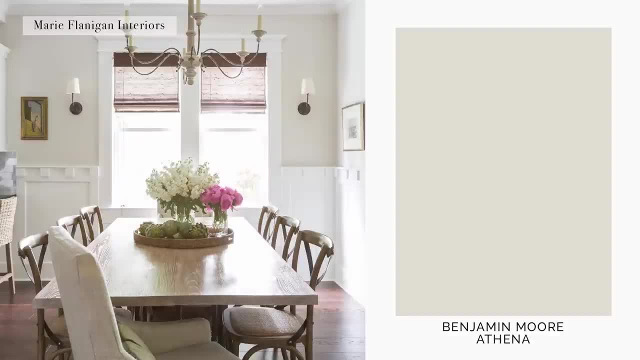 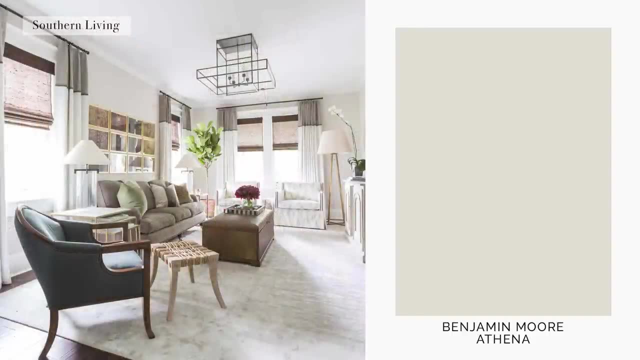 just a little pop on the top or a little pinkish color will bring the feel of the piece straight to your heart. Use this. you can pair as a blue or a white vibe harsh blue or with a white finish. These go well with neon yellow colors. 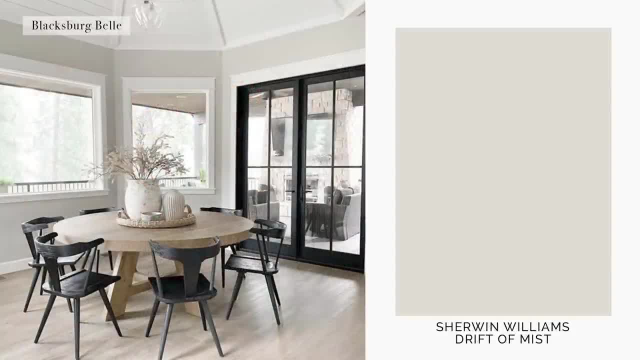 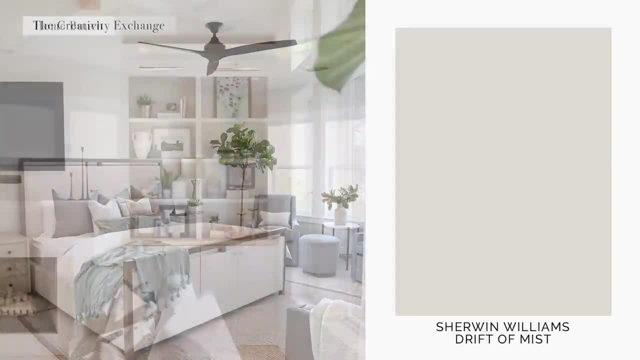 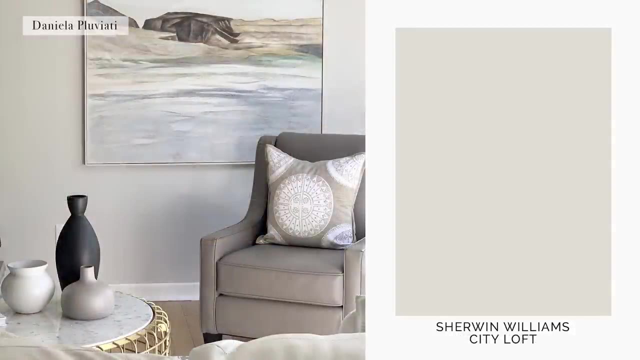 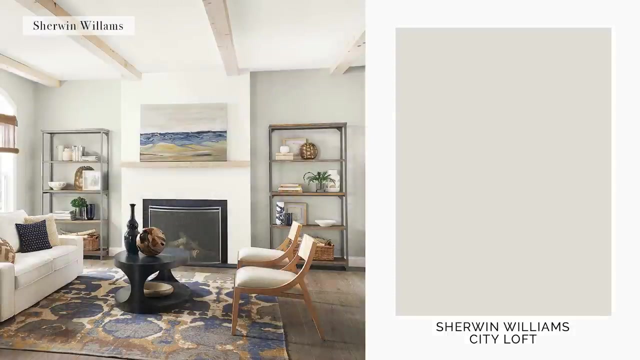 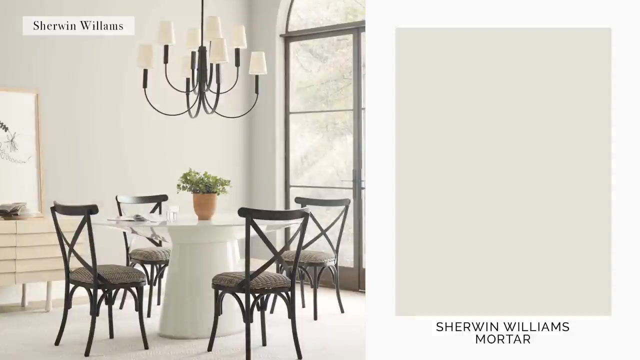 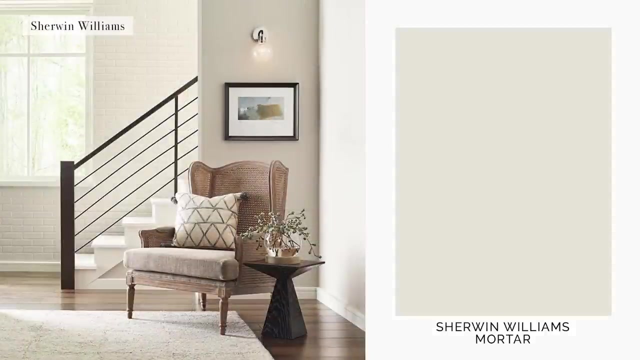 a soft and a light pink tone. Last but not least, a shade of an orange color will make a nice dark brown tone. A dull orange color will add that extra touch and the blue shade will remind you of the summer. Thank you. 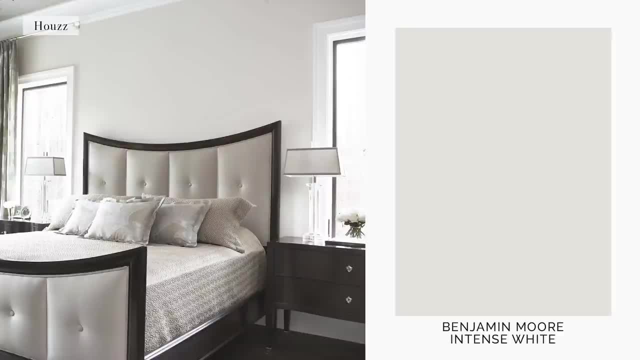 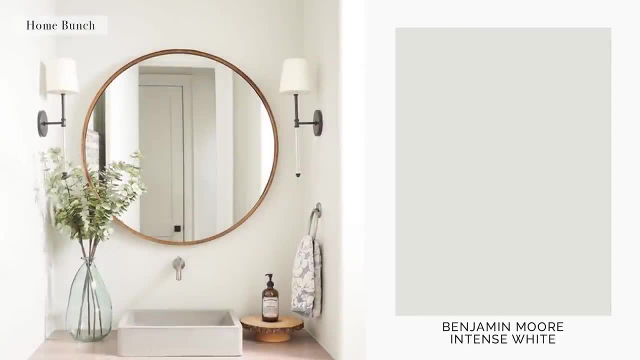 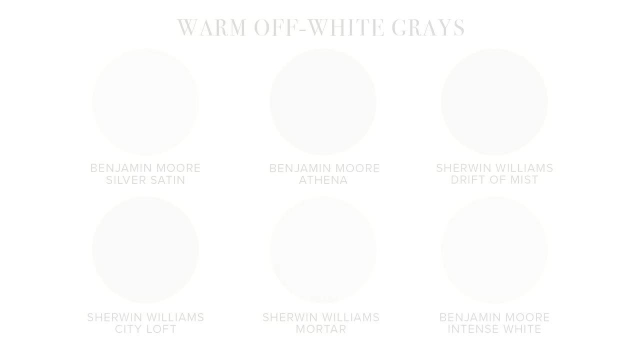 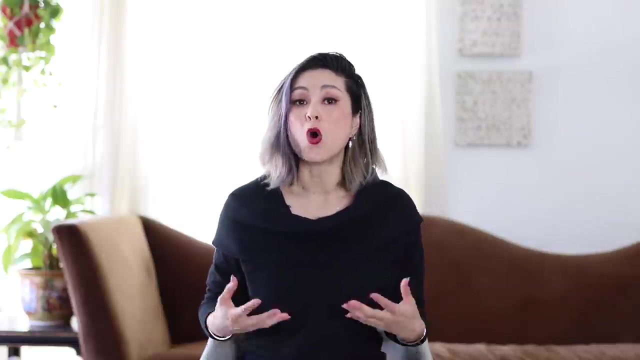 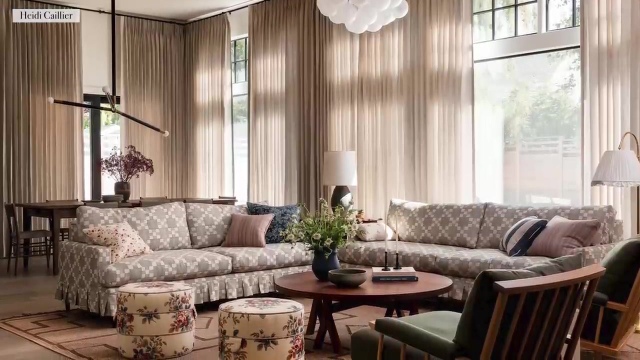 Thank you. Moving on to warm off-whites, Sometimes warm whites and creams can have a little bit too much yellow in them or, in cavernous spaces, can often read cold. So these warm off-white hues are my favorite. They're my favorite to create a cozy spence of calm and relaxation. 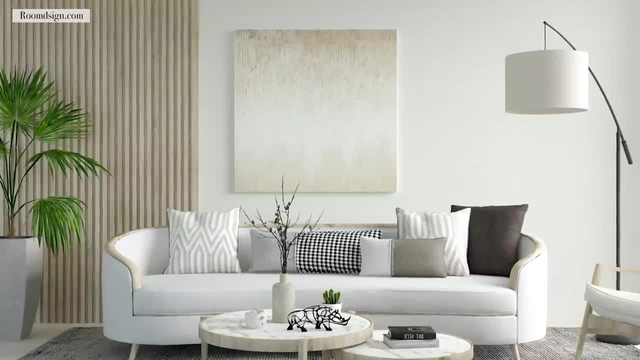 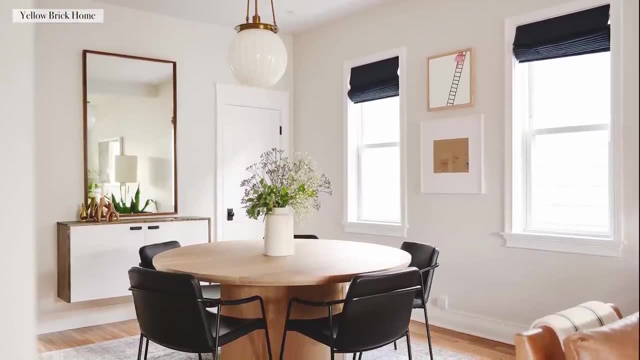 They feel elegant, refined and allow furnishings and art to take center stage. Warm off-whites look great with natural materials like linen, wool and wood. So if you have an affinity for these finishes, these warm off-whites might be the best paint color choice for you. 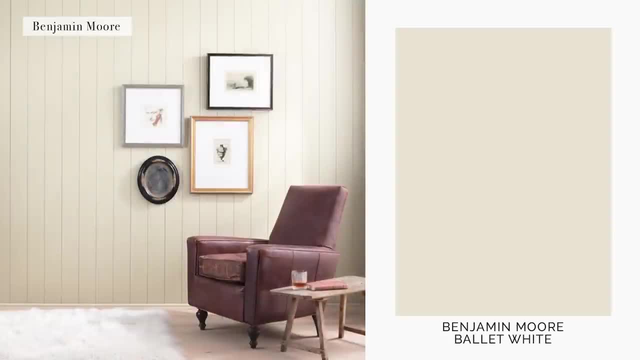 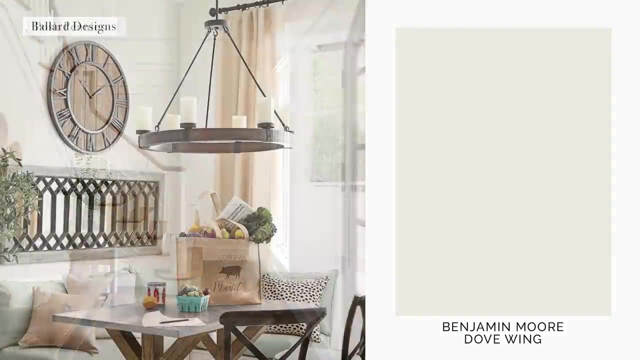 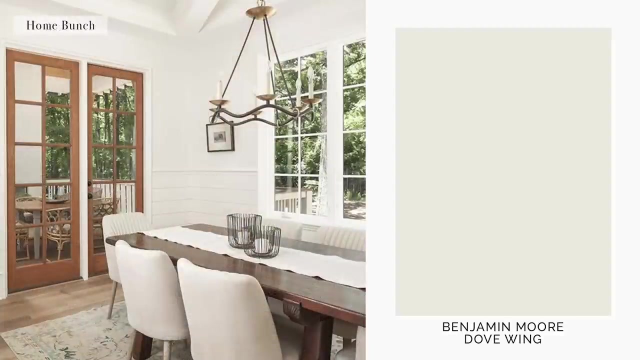 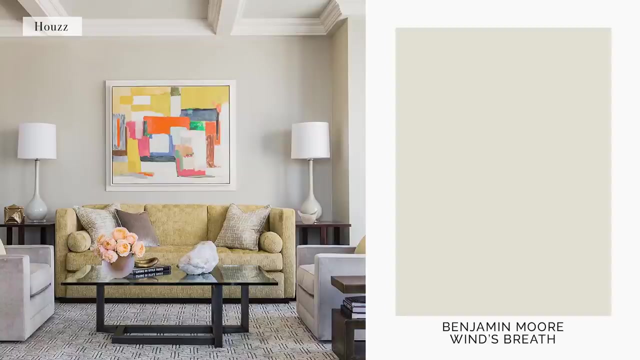 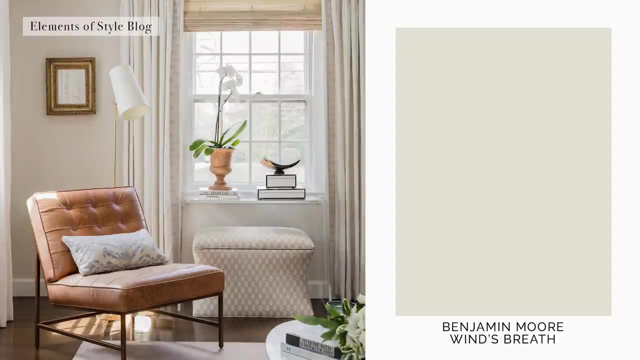 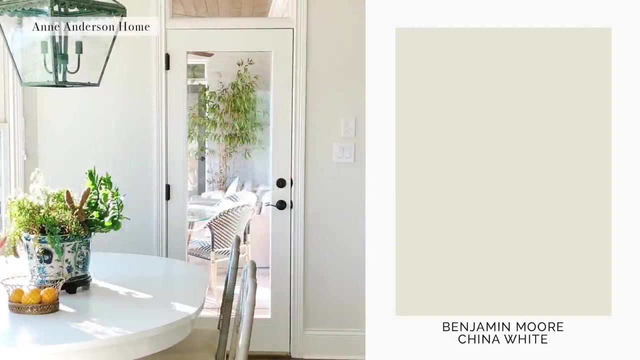 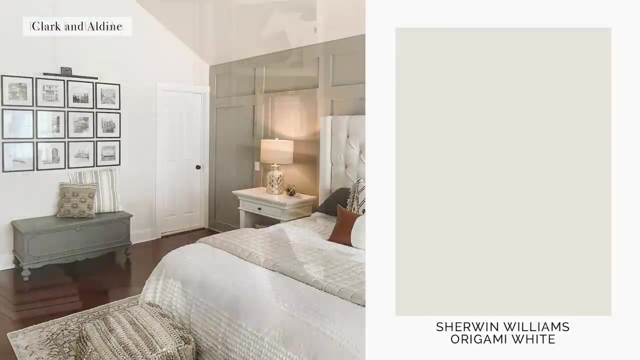 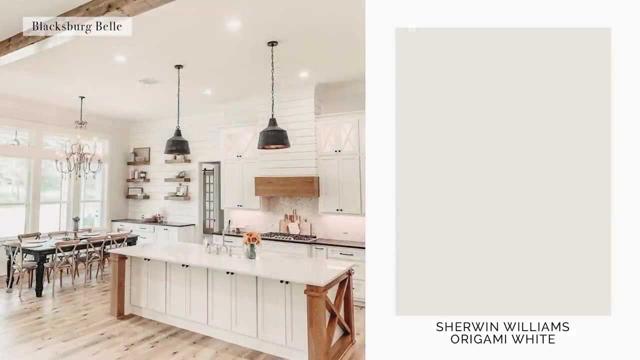 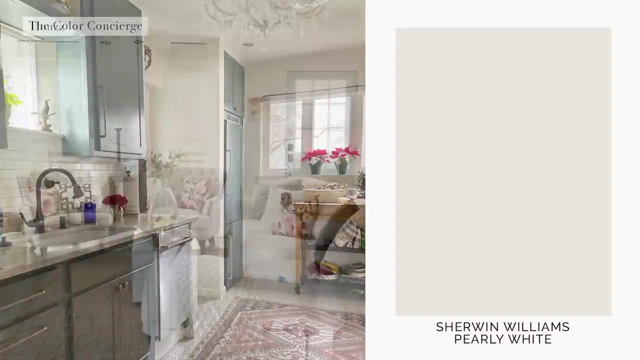 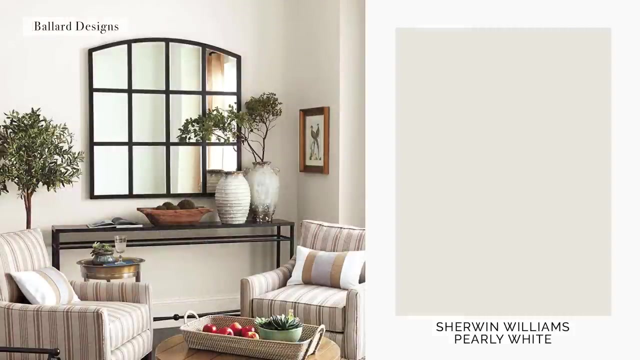 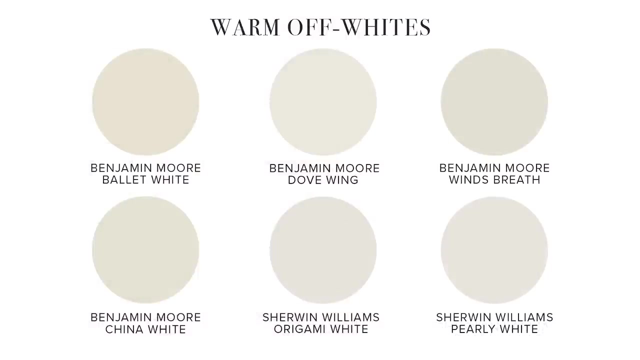 Warm off-whites are great for adding depth and balance to your finished look. Warm off-whites will help you keep your mood strong, as they're really comfortable to work with. They'll also help you get rid of 모. Thank you, Moving on to light to medium taupes. 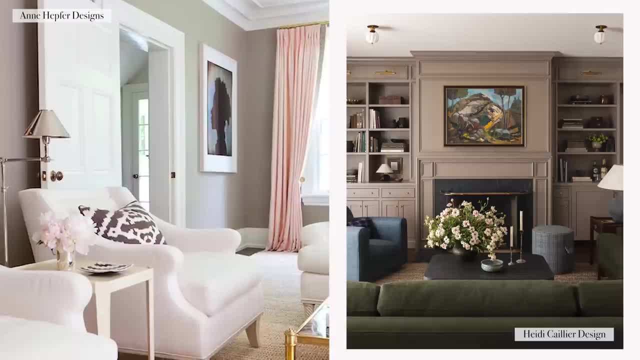 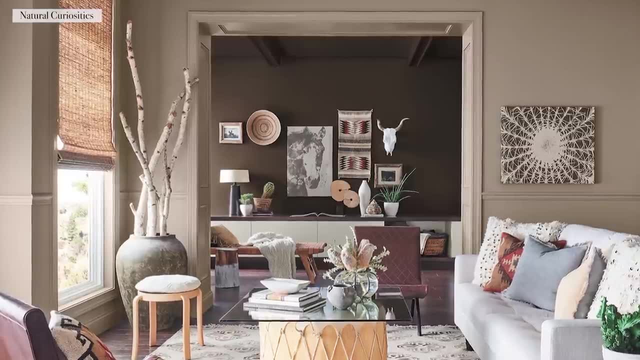 Taupe is typically a darker gray-brown color. They can have a mix of black or red with yellow and green undertones. These pink colors actually favor a purple undertone. So if you've been looking at all of my previous examples and you still feel like the colors are much too warm for you, 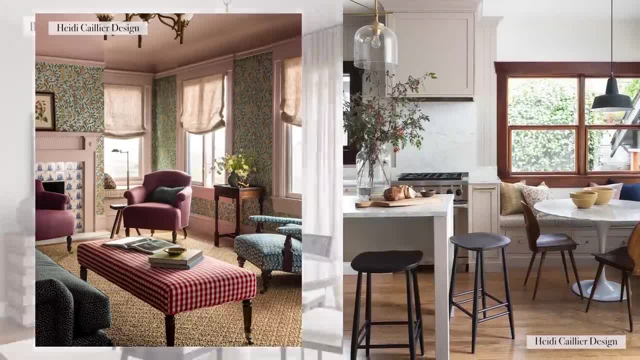 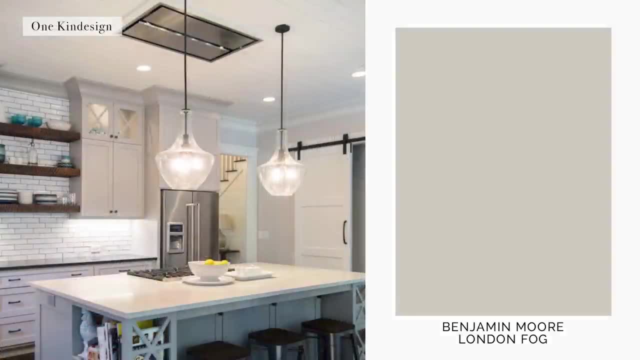 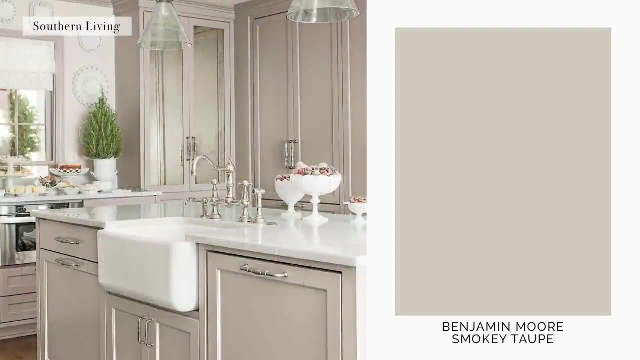 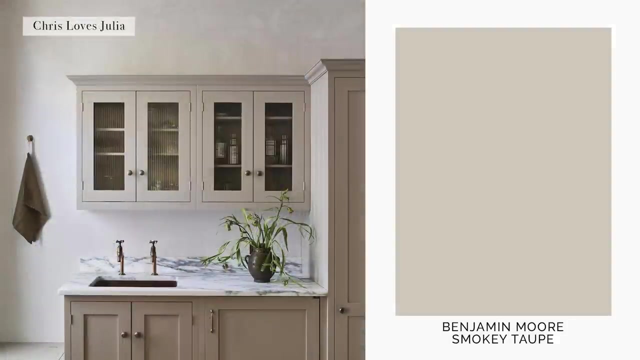 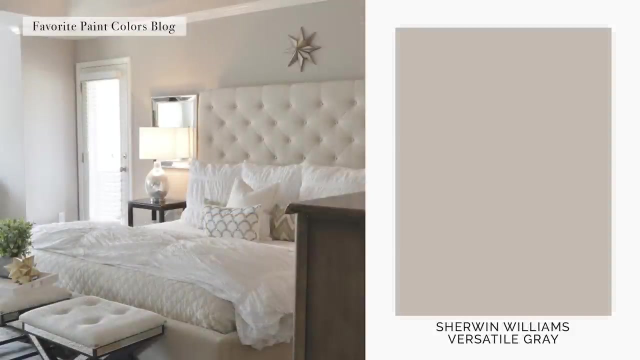 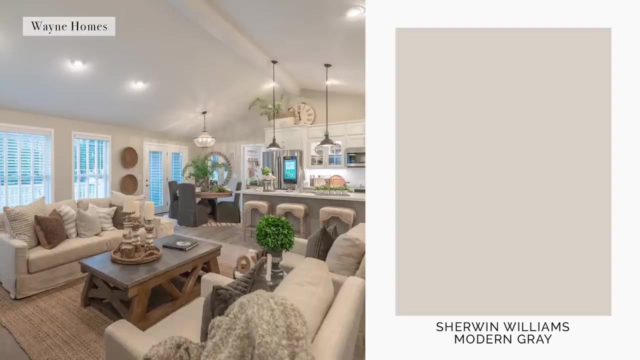 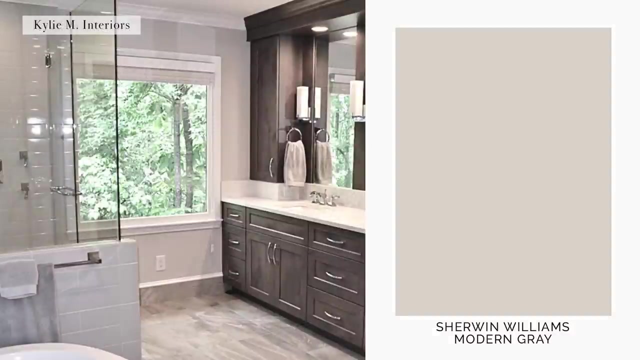 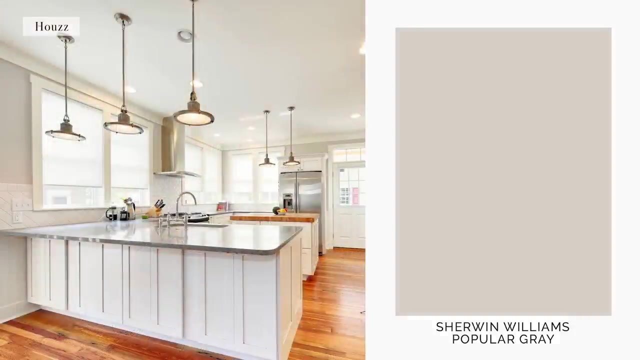 light to medium taupes might just be the neutral you're after. Light to medium taupes is more of a gray brown or light blue. So if you're looking at all of my other videos or other taupes, this is the one you're going to need. I'm going to be showing you what I're going to use to light those colors on the taupes. So if you're looking at all of my other videos or other taupes, I'm going to give you a chance to use these colors. 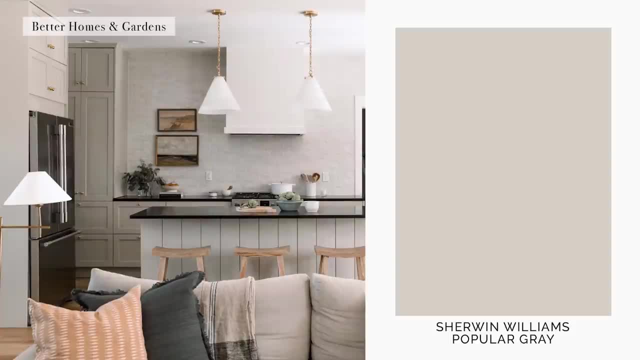 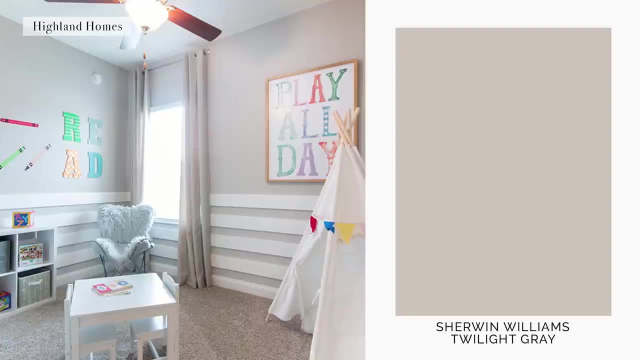 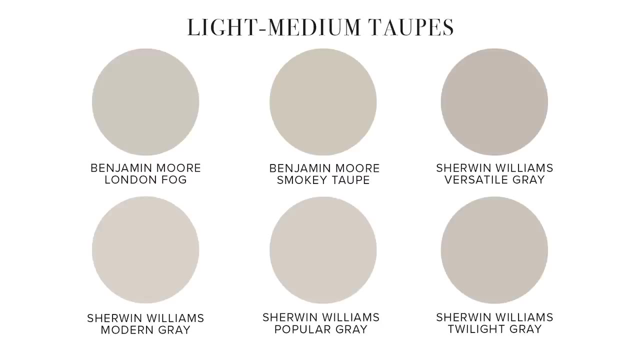 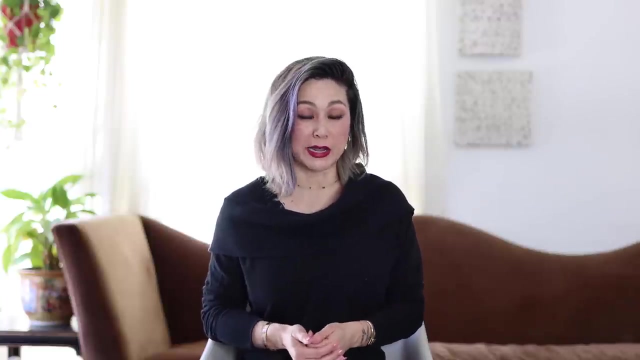 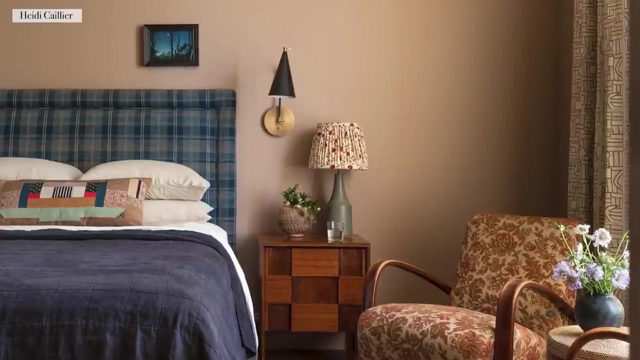 let's talk about light beige. beige might be the most popular paint color for 2023, but there are so many ways to use them so that it feels fresh and timeless instead of trendy and dated. light beige can be described as a pale sandy fawn color, a grayish tan, a light grayish 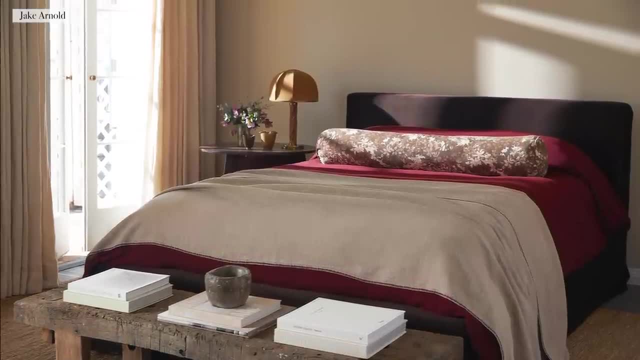 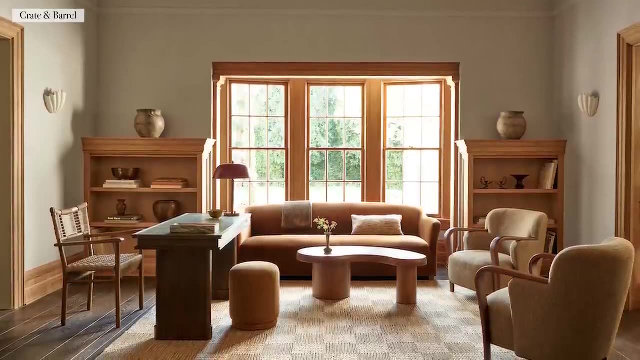 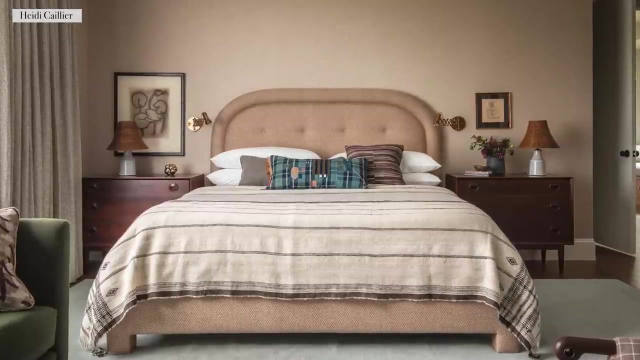 yellowish brown or a pale to grayish yellow. these light beige hues are similar to what we used to specify in y2k, but now updated with more depth and versatility. i love light beige tones paired with rich, dark hardwood flooring, but i can really make a case with light tile as well. 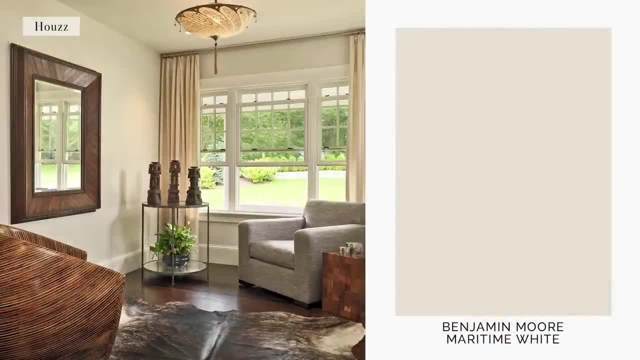 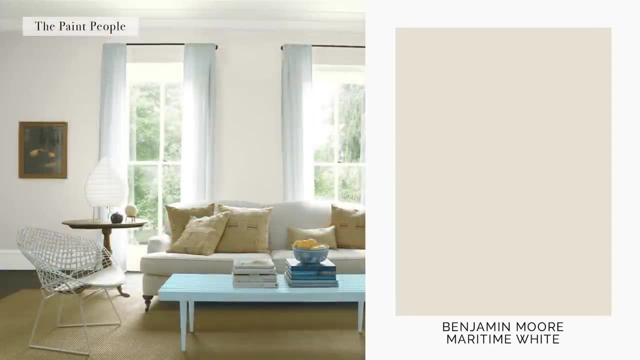 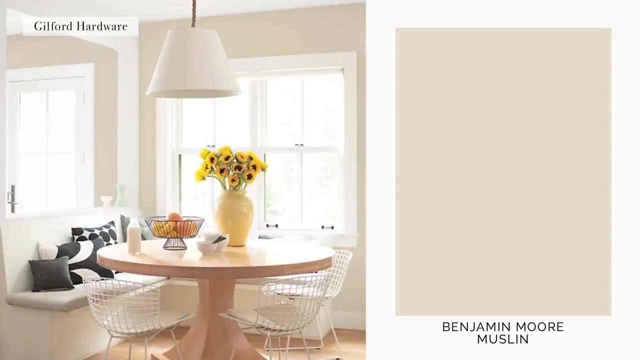 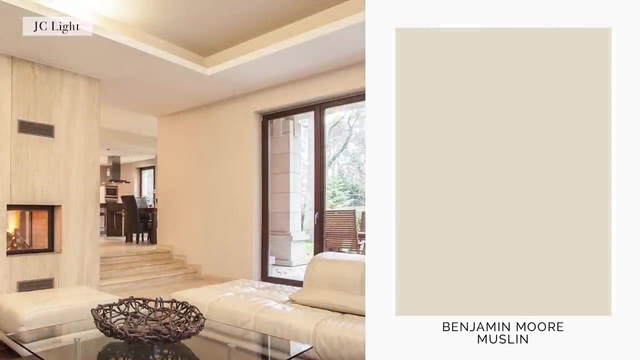 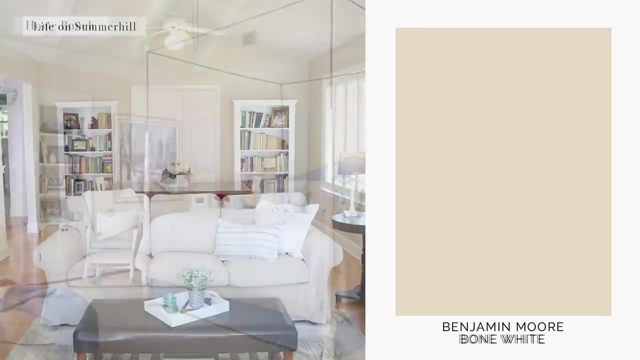 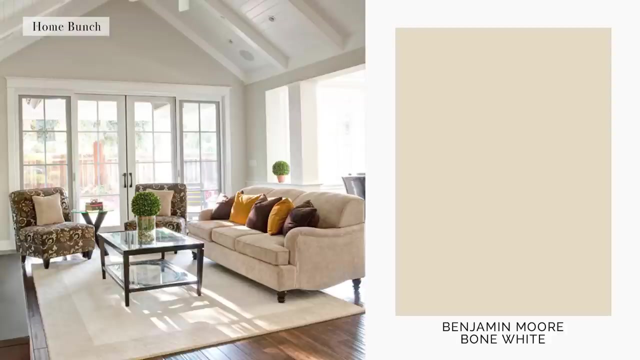 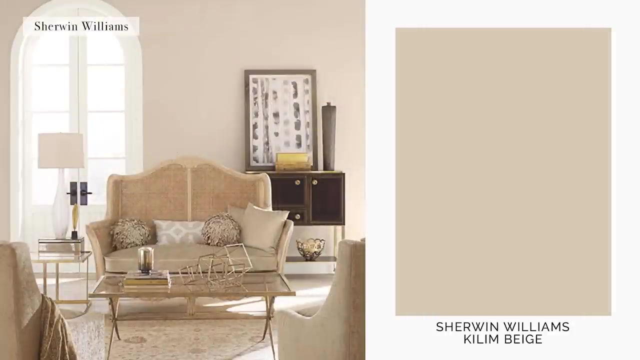 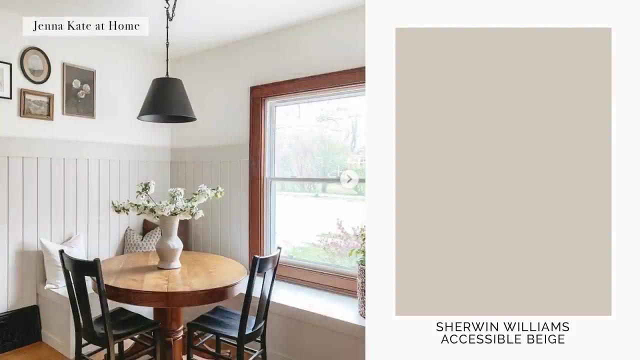 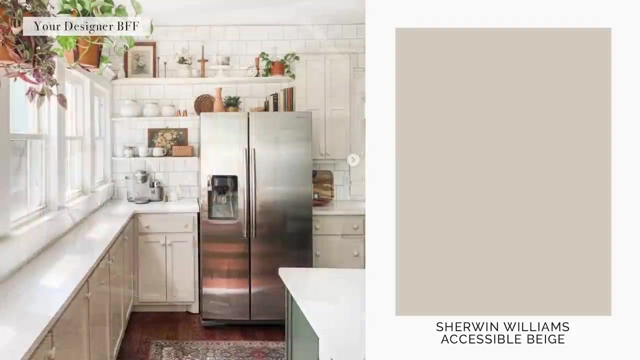 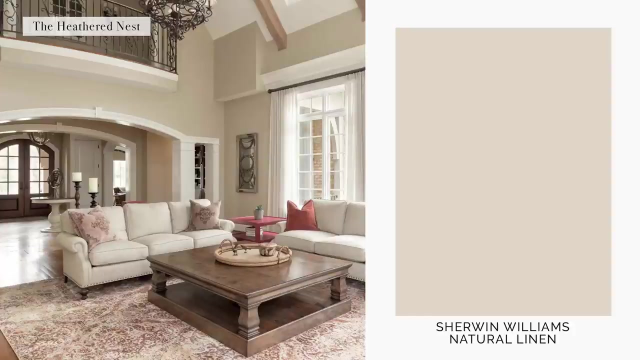 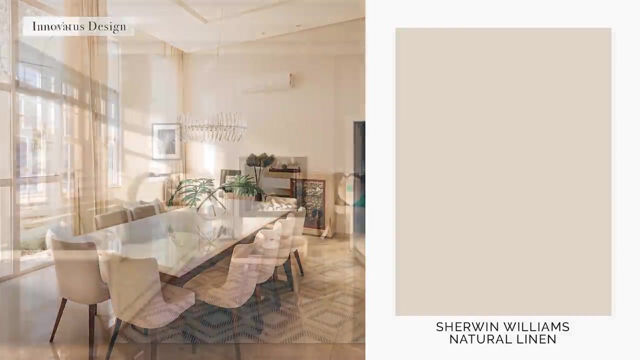 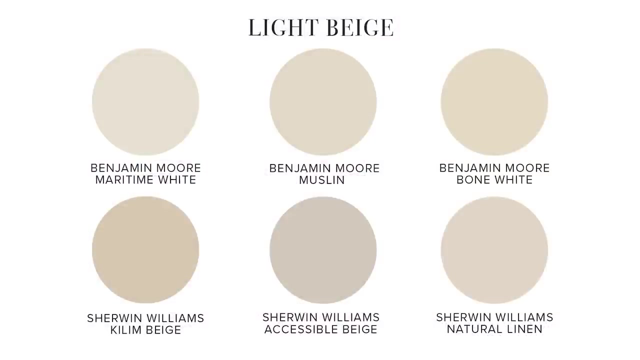 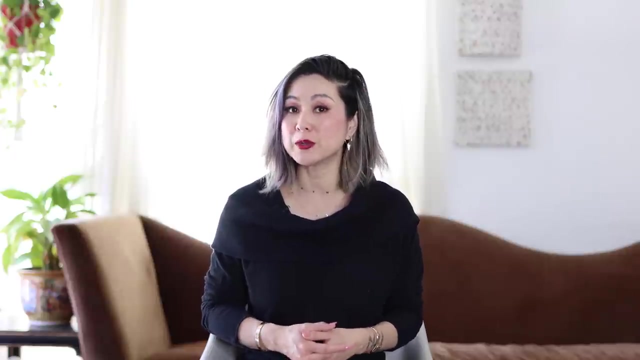 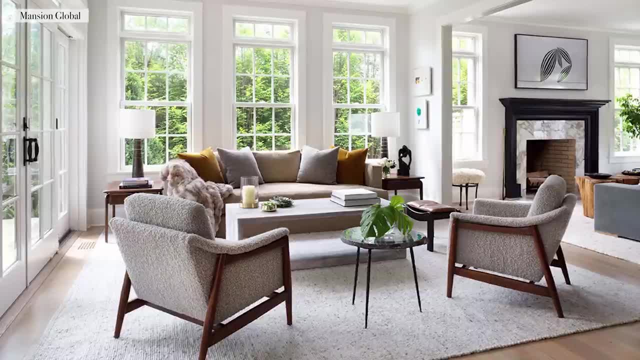 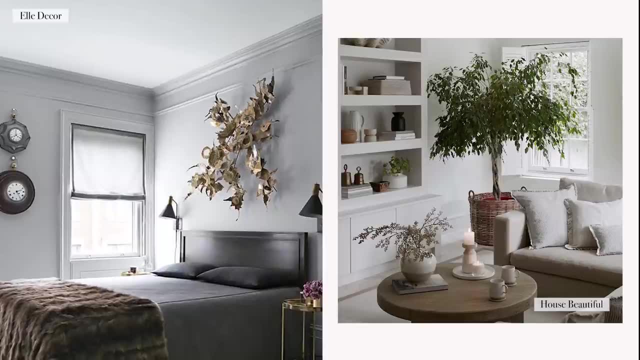 It's perfect for sunlit bathrooms when you want a tint of color, especially against white tile or white countertops. We're not talking about 50 shades of gray from the early 2010s, but my new favorite grays have a touch of cream in them. 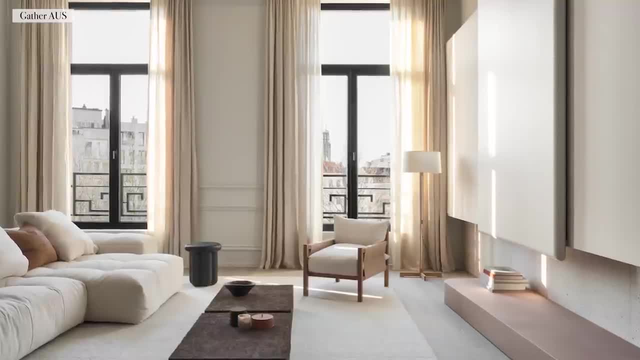 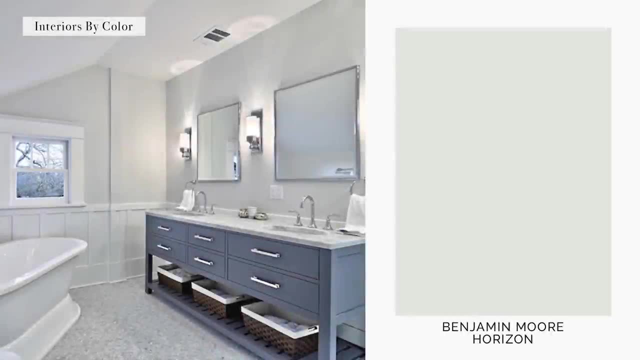 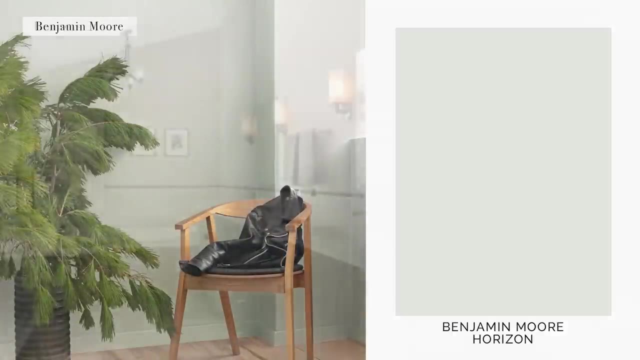 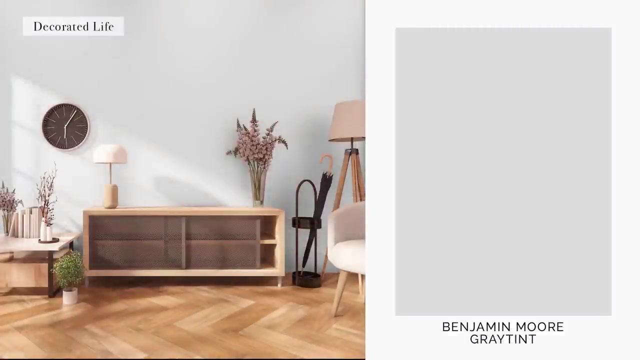 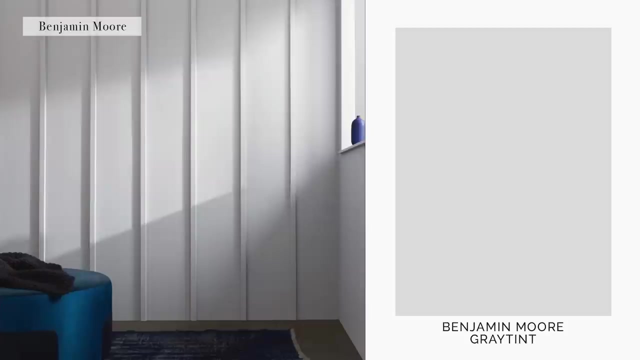 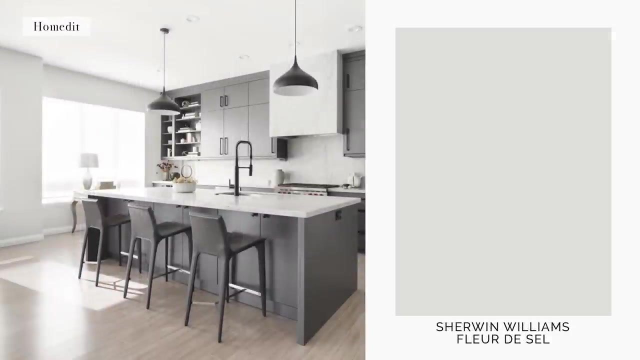 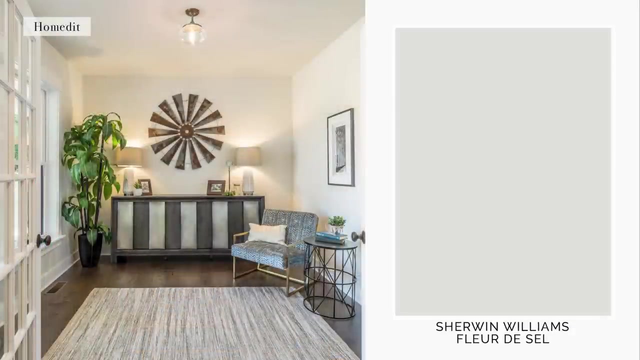 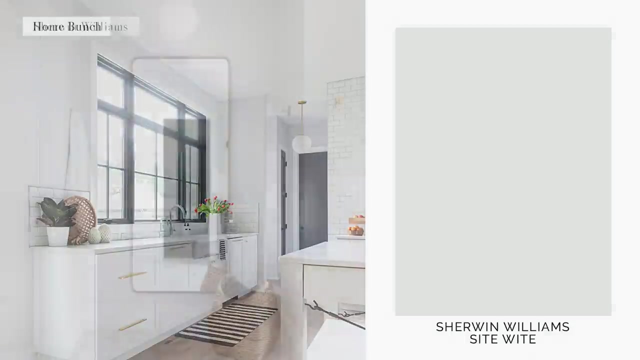 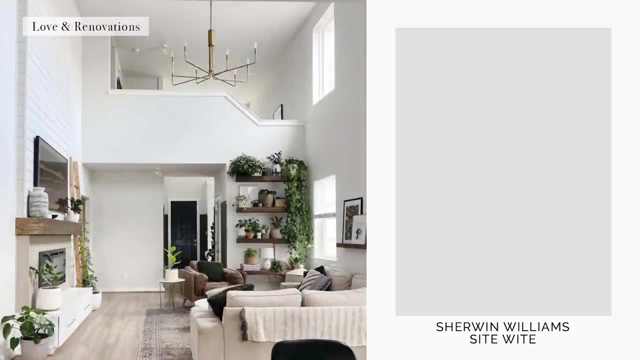 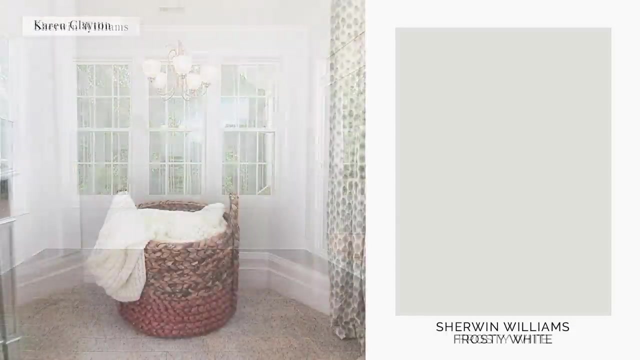 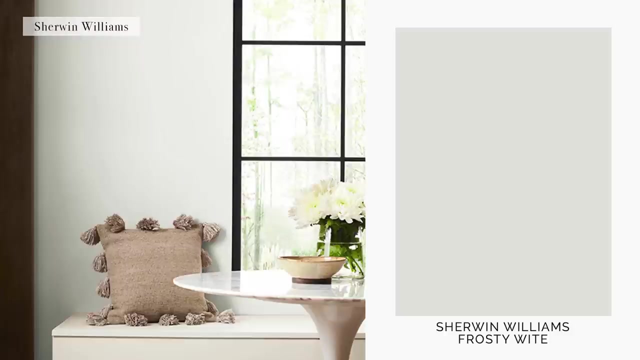 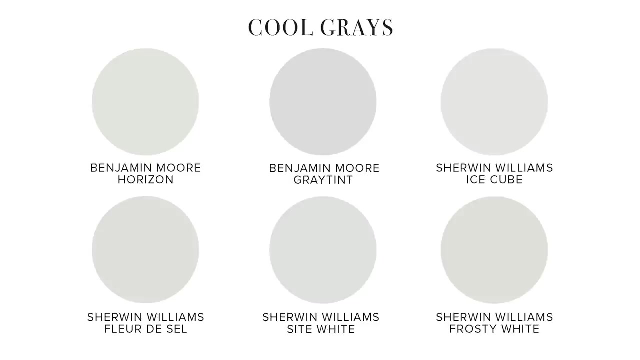 making them just a tad warmer and not so clinical and depressing. But that's all subjective, of course. So check out my favorite cool, neutral grays and let me know what you think. I'll see you next time, Bye. This last section encompasses all of my favorite neutral greens. 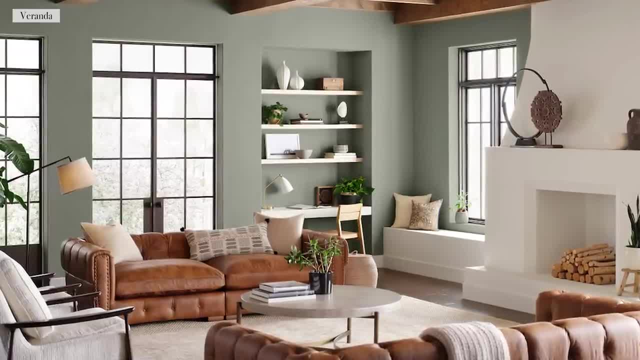 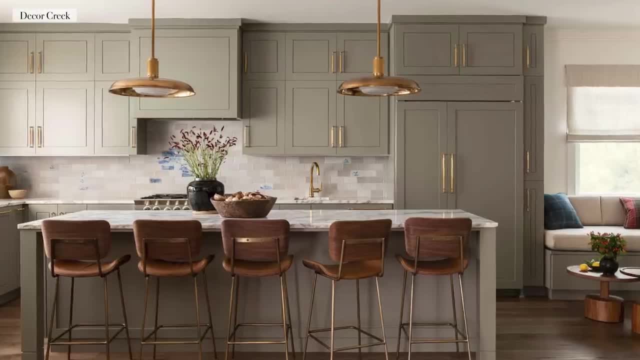 Some of my favorite greens can also appear gray, depending on how it's used. These greens can bring in a coastal vibe to a seaside interior, or even a traditional vibe to a classic cottage. Green has the ability to energize and rejuvenate, relax and calm. 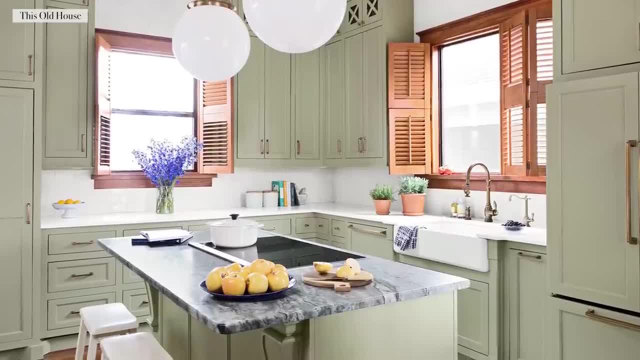 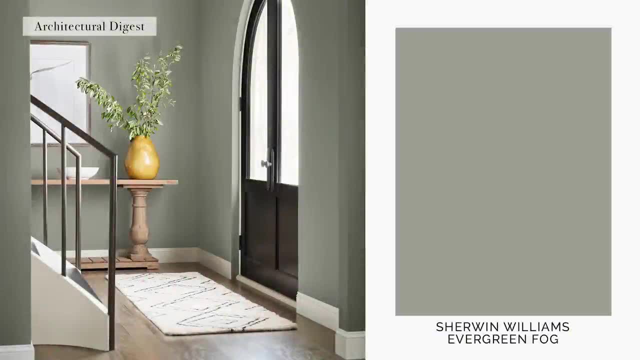 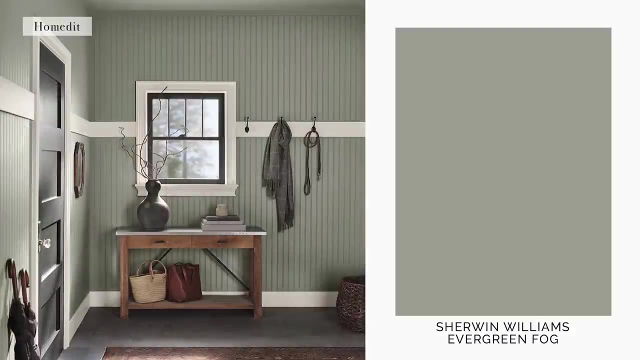 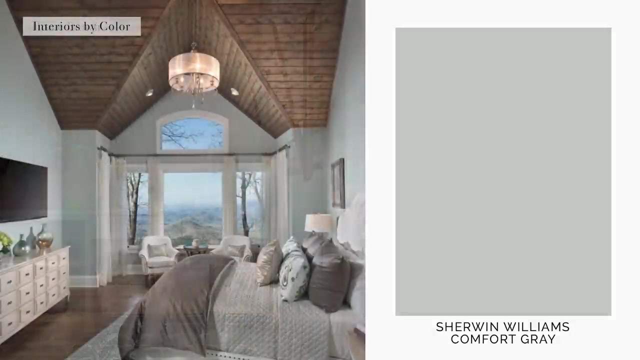 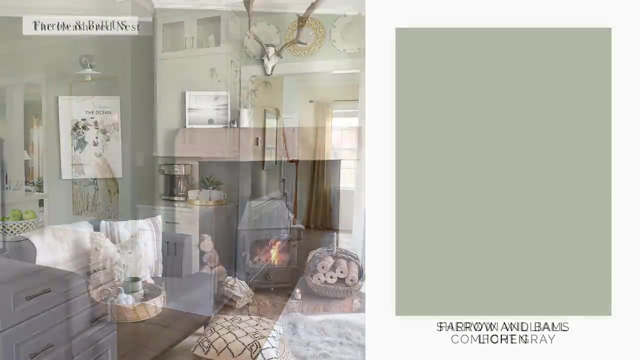 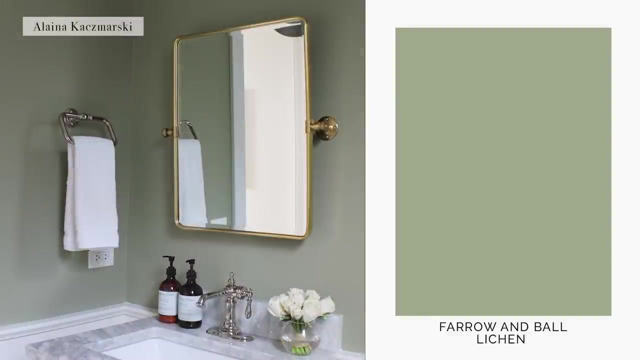 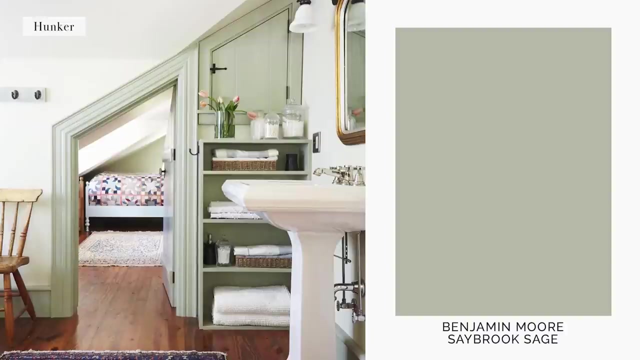 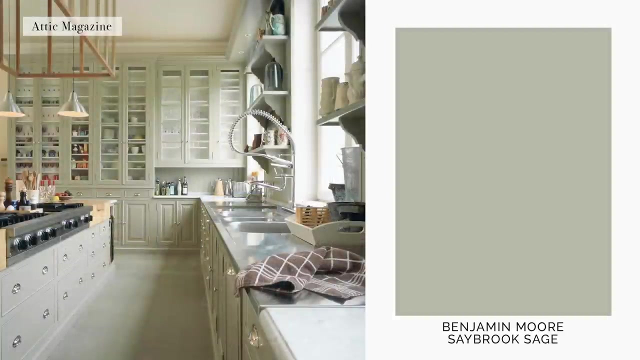 In fact, I'm redesigning my bedroom now and I'm going green Now. I just need to find the perfect shade. Where can you imagine painting a room green in your home? I have goals you can set. We'll talk to you about that in a few minutes. 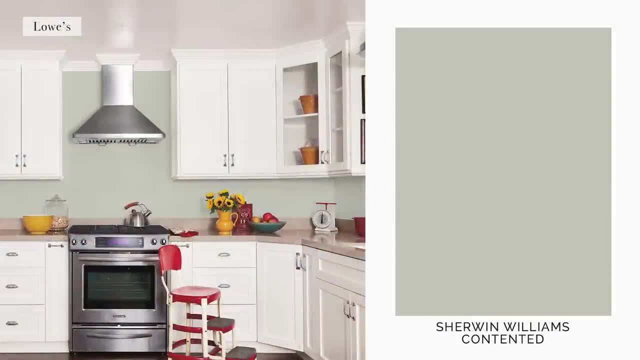 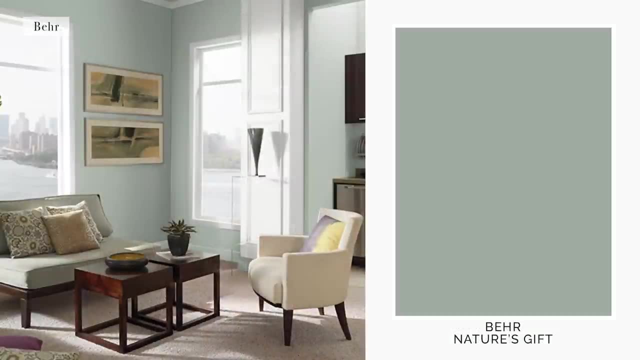 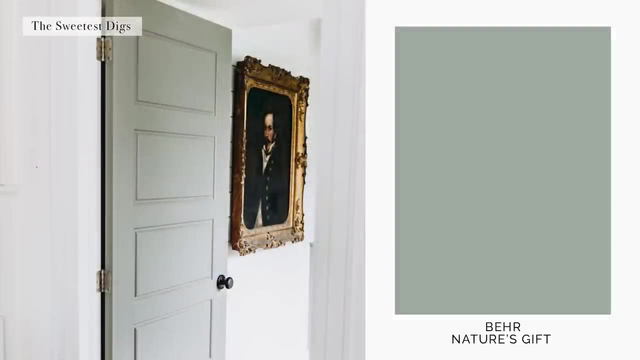 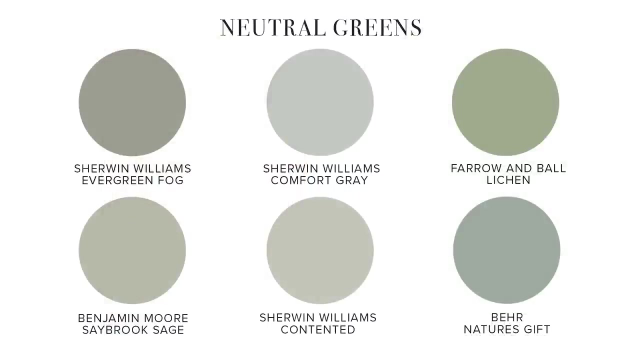 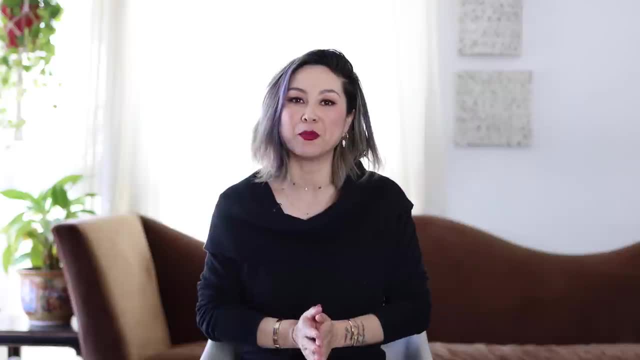 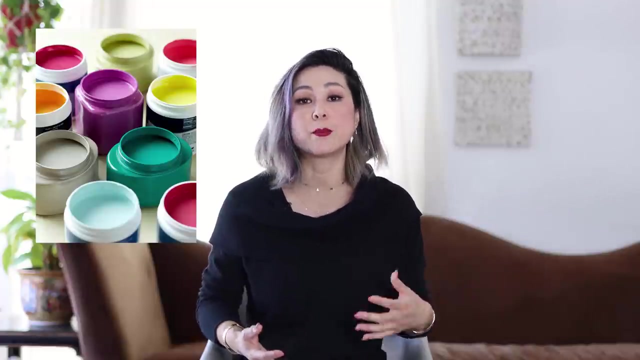 the perfect paint colors for your home. Sample, sample, sample. I cannot stress this enough. If you've watched any of my paint videos, you will know that I always talk about sampling. There's many ways to sample paints. A small pot of paint sample can cost you anywhere between $5 to $10. 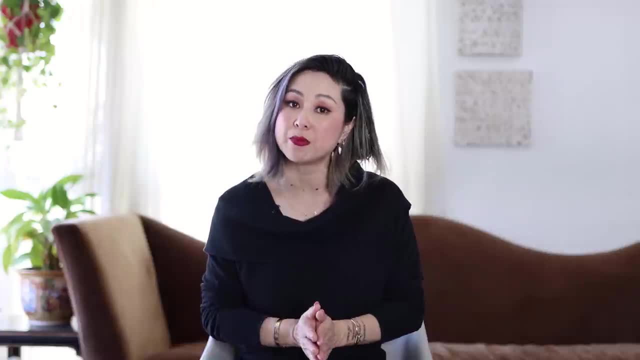 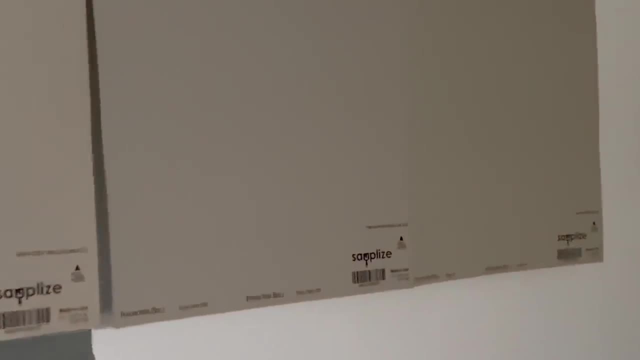 You can purchase this in store. You can purchase this straight from your paint manufacturer's website. You can also purchase removable peel and stick paint samples from vendors like Samplize. I actually use them often. They're so easy to use without all that paint mess. 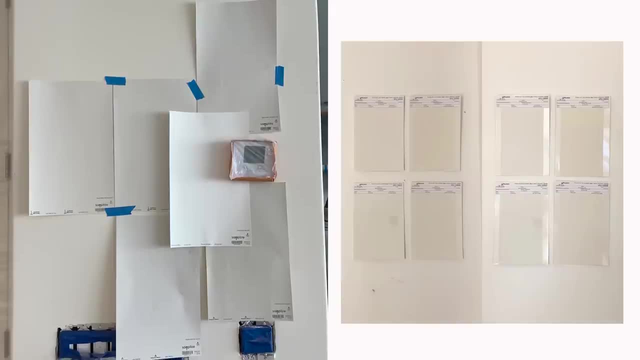 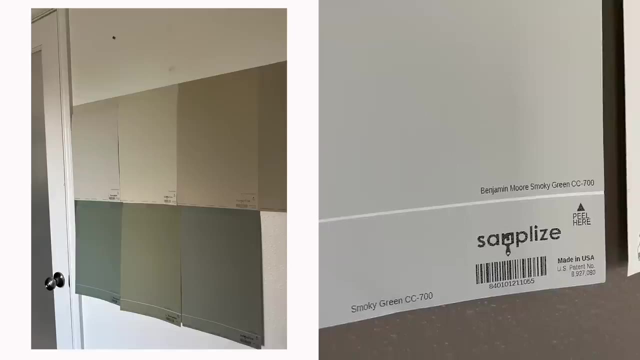 They only offer specific brands and their colors are limited, so choose a route that's best for you. Remember that the furniture that you already have in your space, the specific time of day or even the type of light source you have can greatly alter how the paint color appears. 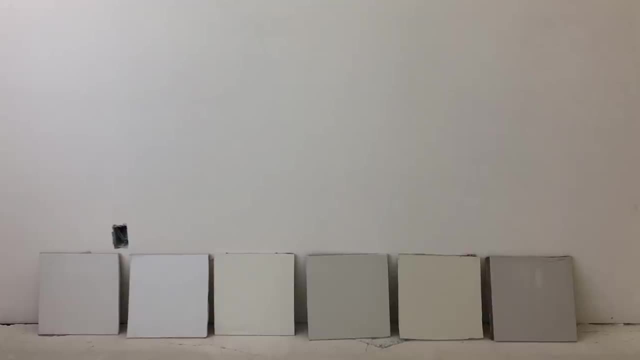 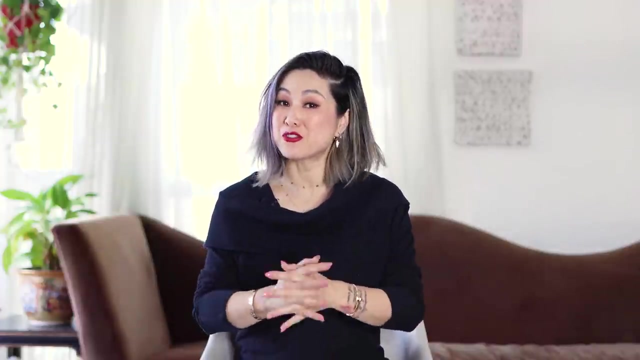 So, before you take the plunge, make sure that you see large samples of color on every single wall in your room at all times of the day. That's it for today's video. What did you think of my new video? What are your favorite neutral paint colors? 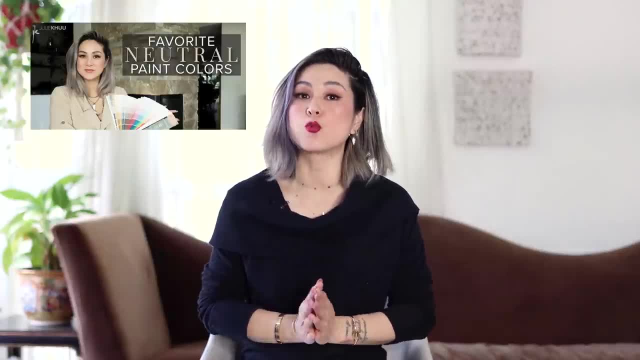 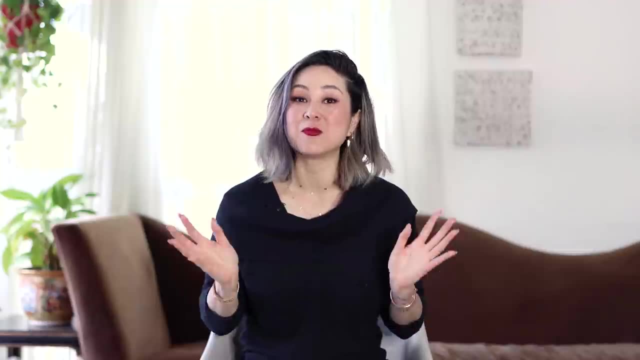 Make sure you watch my previous video on best neutral paint colors, where I share over 65 of my favorite neutral hues. A lot of those neutral hues have not changed. This video is just to supplement the previous video, but there is so much information jam-packed. 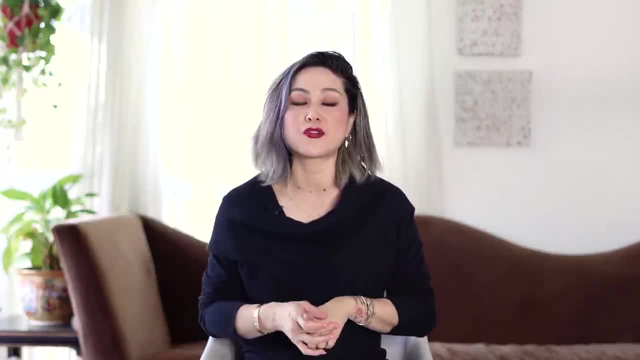 in that previous video, including how to choose the best sheens for every single room in your home, I break down some of my favorite paint brands, the differences between each brand, including the application, The cost, how you apply it in different rooms in your home and even how to pick the perfect.